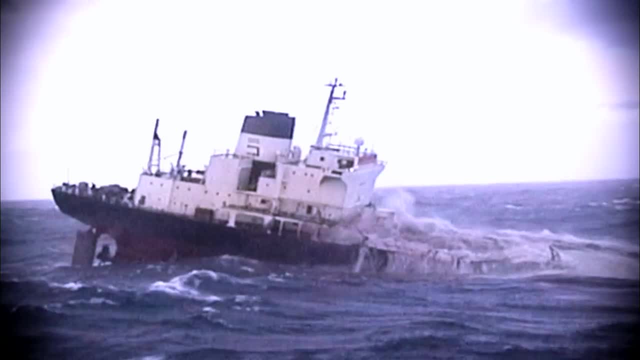 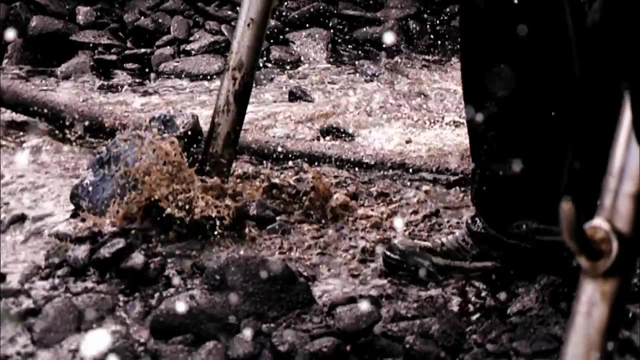 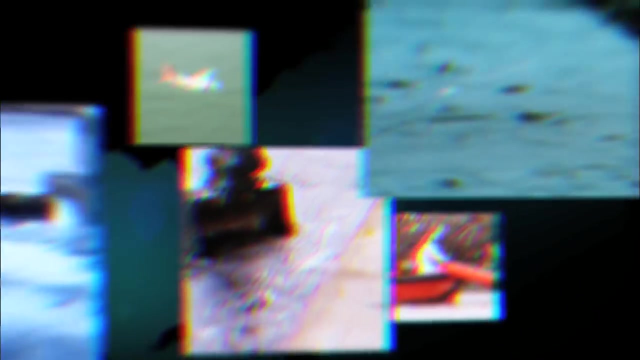 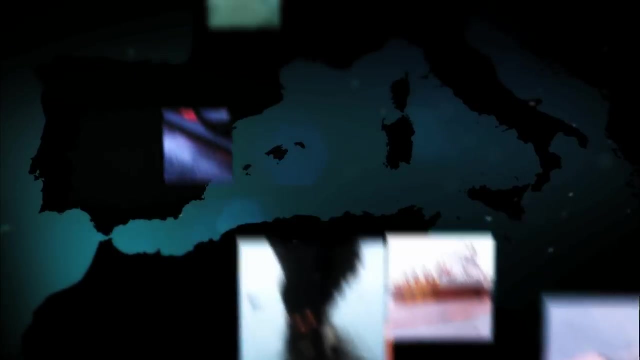 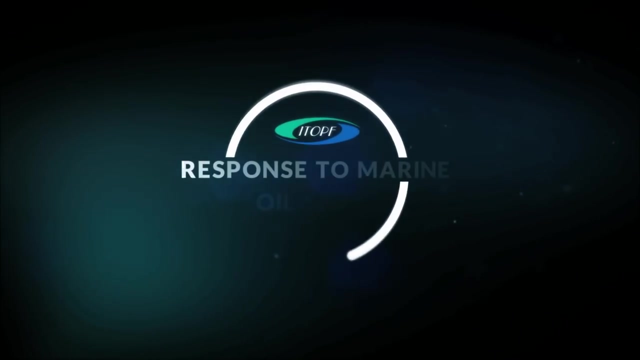 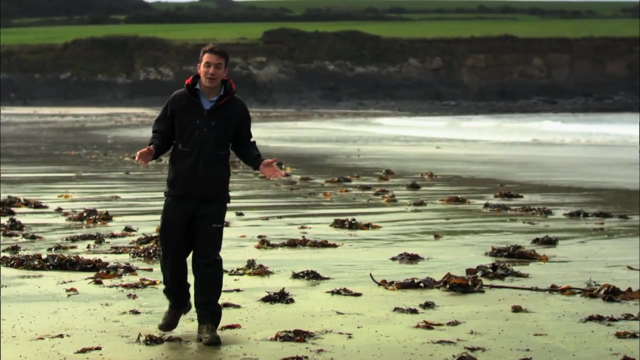 What issues do we need to consider, What expertise and techniques are available And how do we deliver a well-planned and executed response to minimise impact? In this film, we'll be looking at some of the first things to consider when planning a response. 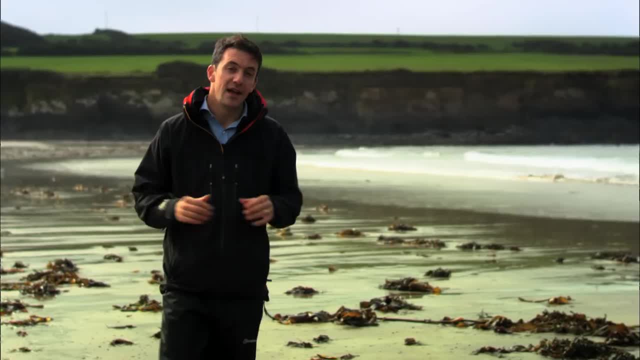 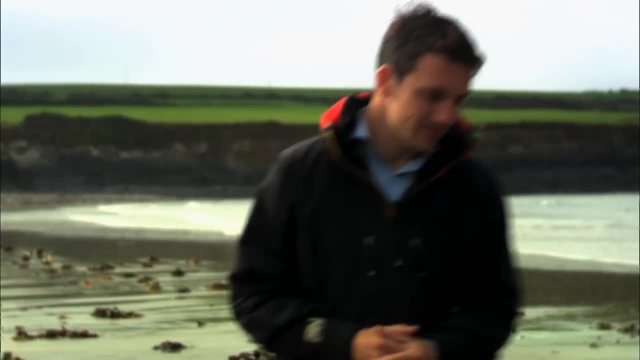 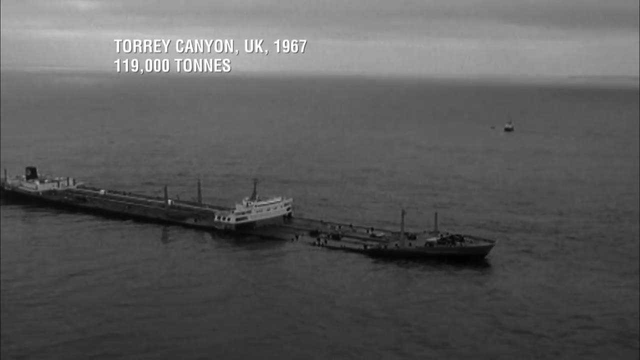 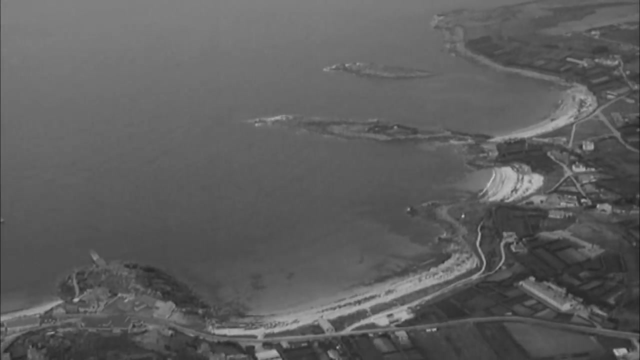 In particular how different types of oils behave in the marine environment. But first I'm going to find out a bit more about the history of oil spill response, The giant tank at Torrey Canyon, a ground off Land's End. In 1967, the world watched as the Torrey Canyon tanker spilled 119,000 tonnes of oil. 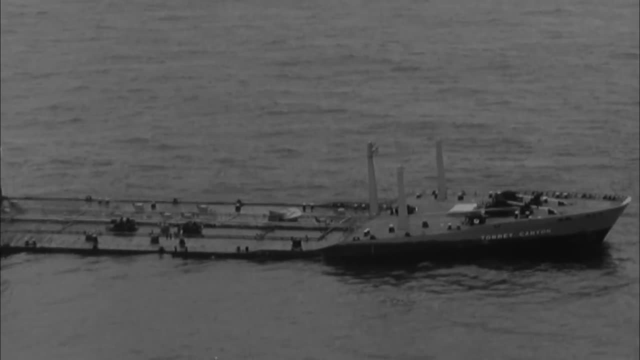 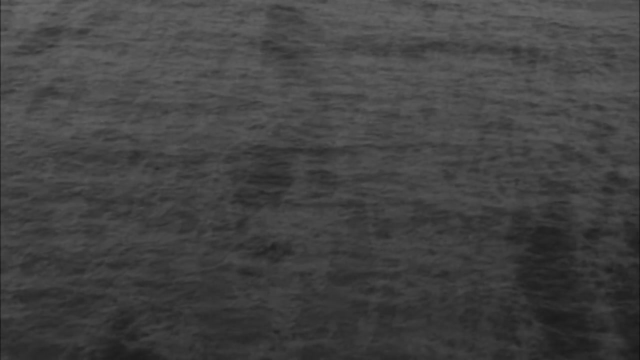 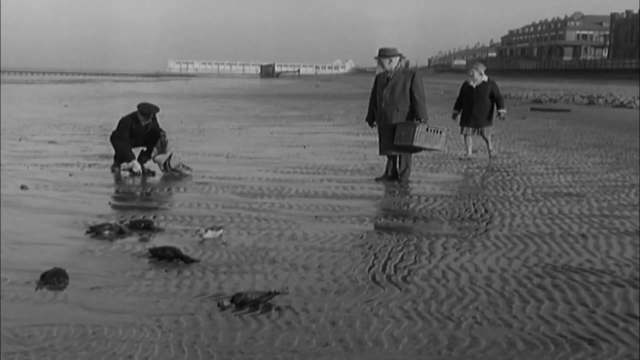 into the sea. off the UK coast, On the Seven Stones Reef, 16 miles off Land's End, she lies like some stranded ocean monster, shedding her life blood. The impact was widespread, threatening livelihoods and resulting in the death of thousands of seabirds. 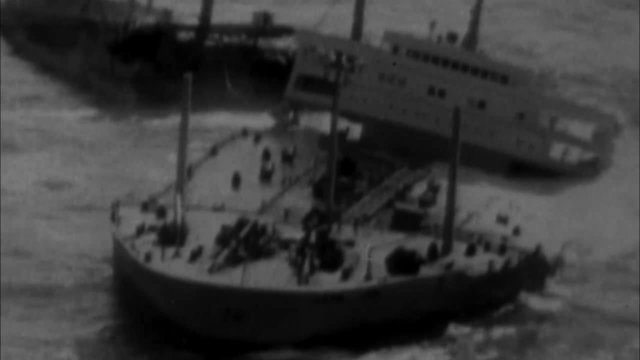 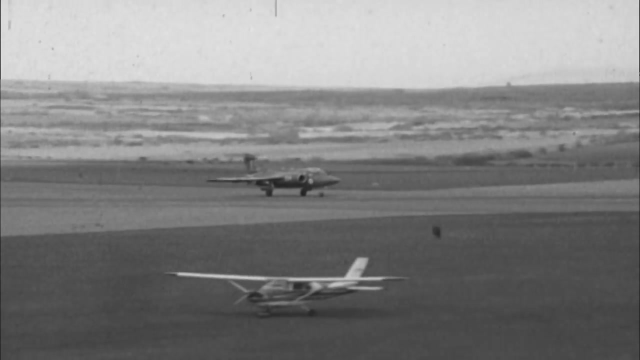 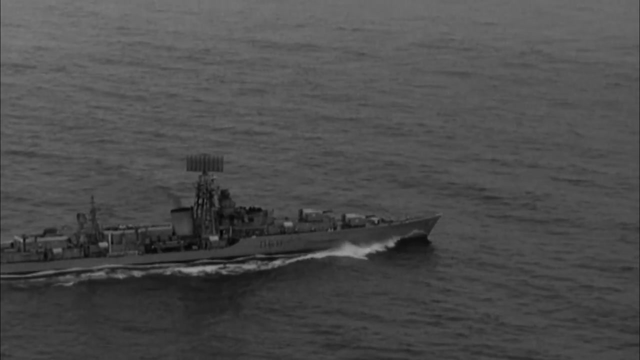 At the time, the Torrey Canyon was the biggest ever oil spill and the first involving the new breed of supertanker. The authorities struggled to coordinate an effective response And, in some cases, made matters even worse. Naval vessels joined the dispersal fleet which was shadowing the slick. 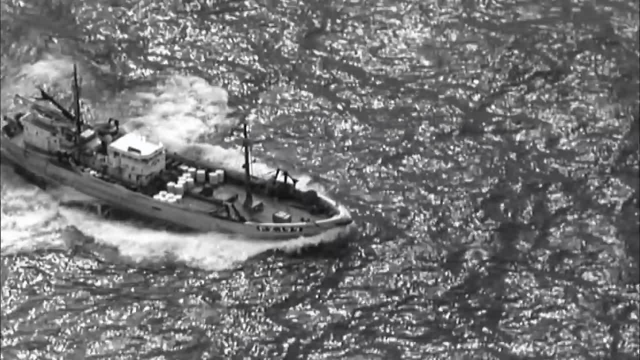 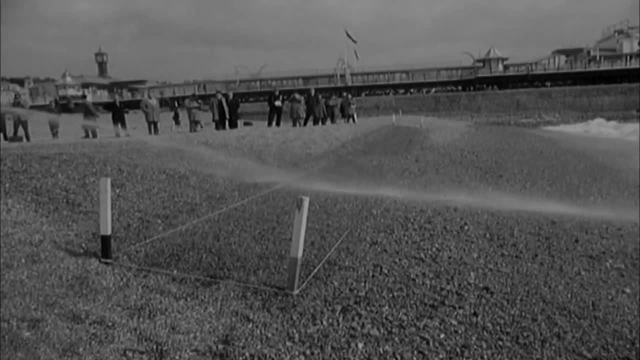 and bringing in thousands of drums of detergent to try to break it up. The know-how for dealing with spills on this scale simply did not exist. Surely it's time there was an international effort to beat the menace before it gets completely out of hand. 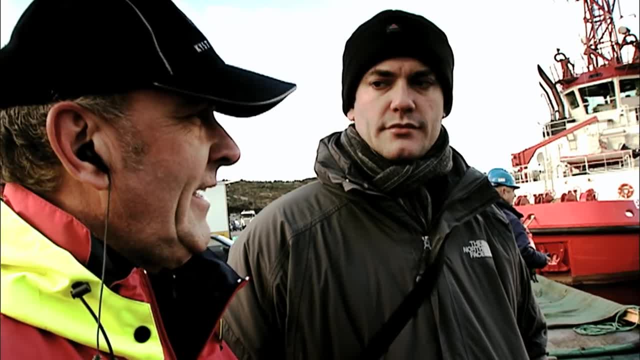 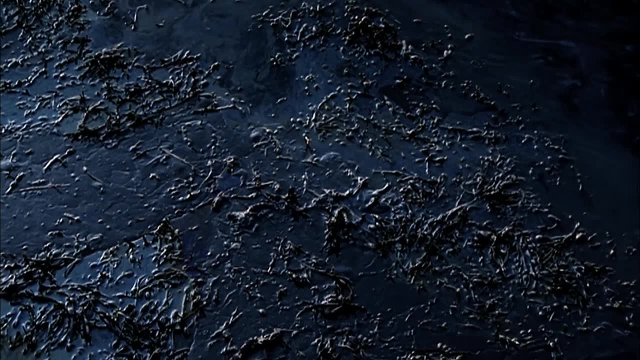 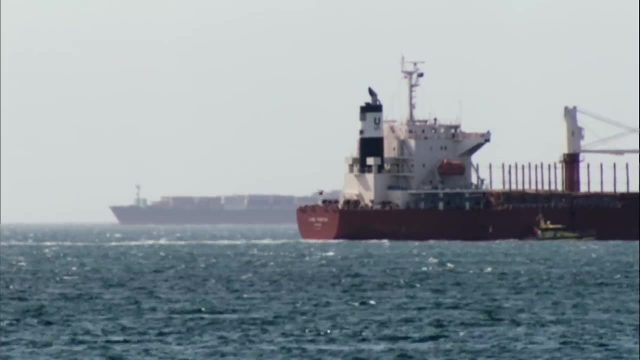 In operation since 1968, ITOF is now the maritime industry's primary source of objective technical advice about marine spills of oil and chemicals. Set up in the wake of the Torrey Canyon, it's a not-for-profit organisation funded by the shipping industry. 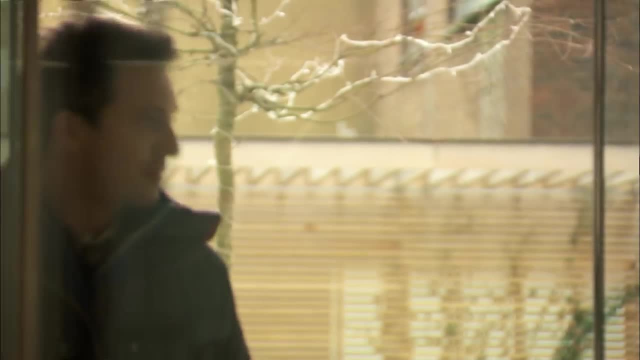 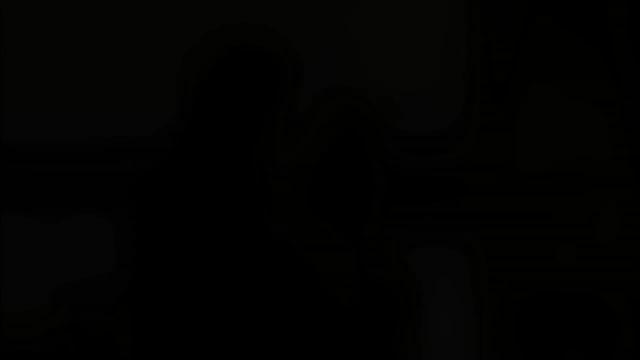 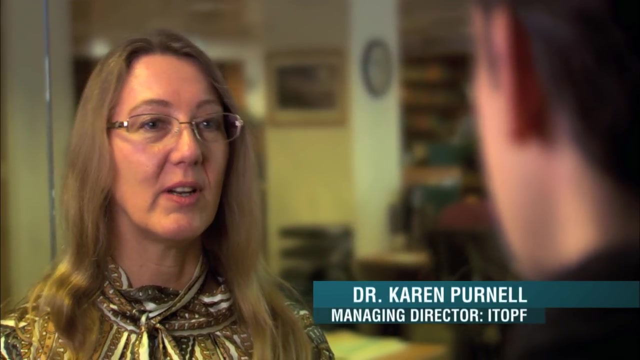 I want to find out what they're all about, So I'm visiting their headquarters in London to meet with Managing Director Karen Purnell. Karen, tell me about the role of ITOF. What exactly do you do? Well, ITOF provides technical advice on oil and chemical spills. 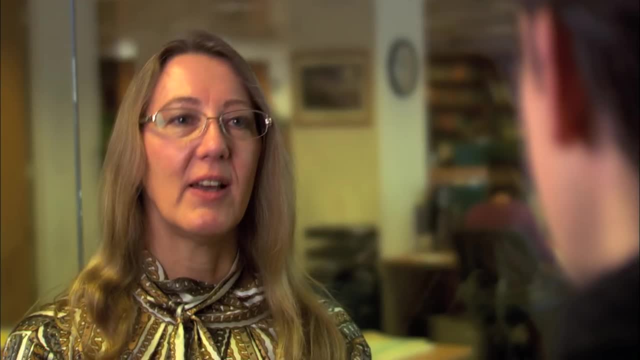 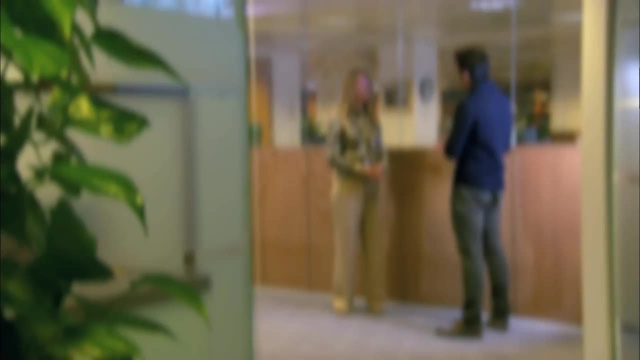 and we provide that to the shipowner and his insurer and also to the local governments, local environment agencies and to all the people affected by the oil spill. And how involved are you in the process? Do you get involved right at the beginning? Absolutely yes, as soon as we get the call. 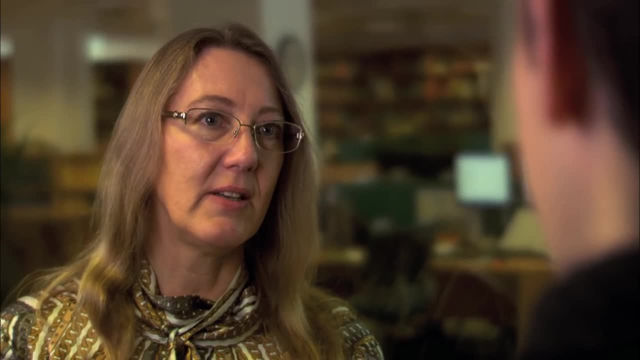 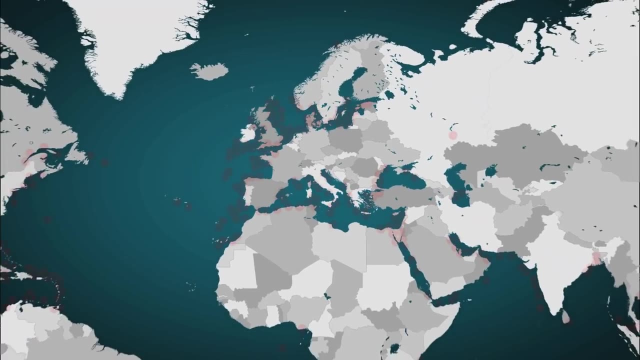 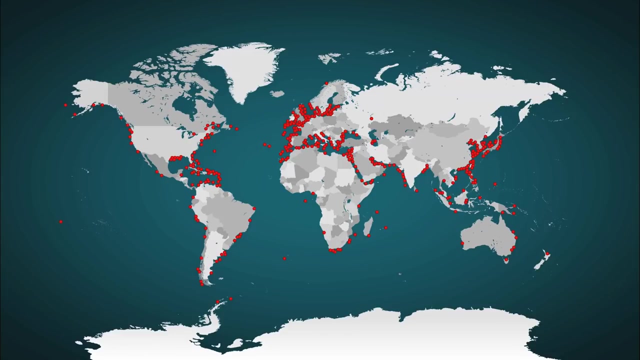 If it looks like it's going to be a serious incident, then we may send one or even two people straight out on the next flight and going to the country and being there as quickly as possible. ITOF has attended hundreds of spills, including all the major tanker spills, in countries around the world. 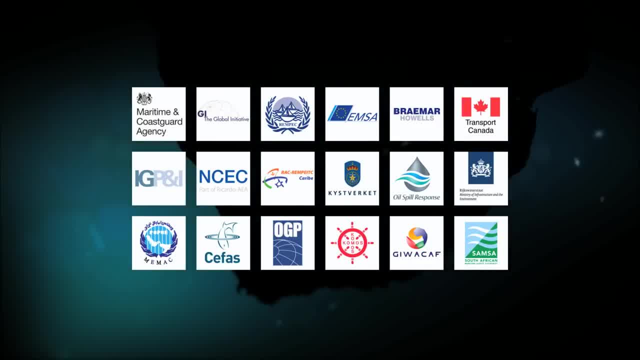 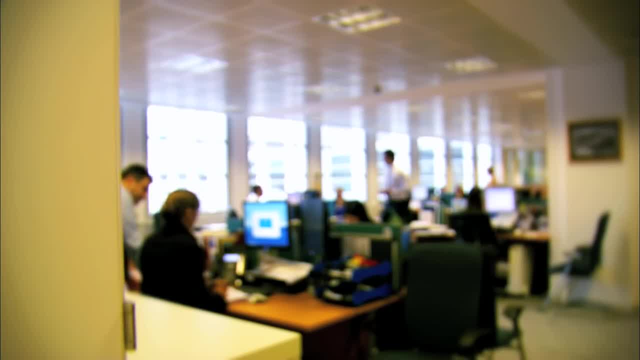 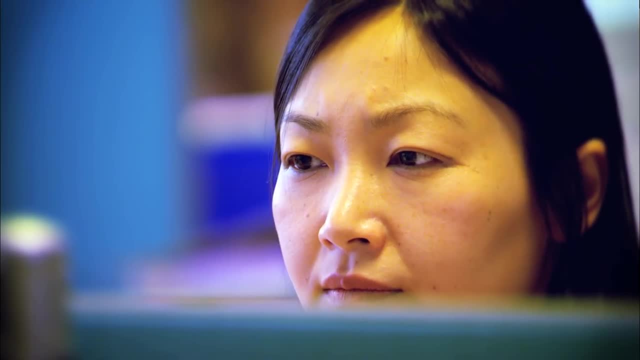 Partnership with the global spill response community has been vital in responding to and learning from every incident, And as well as that experience, you have a tremendous amount of expertise here. What sort of people, what sort of qualifications do you have within your team? Probably the most important qualification is stamina diplomacy. 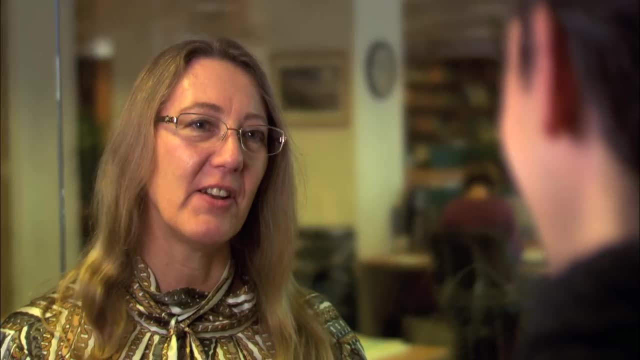 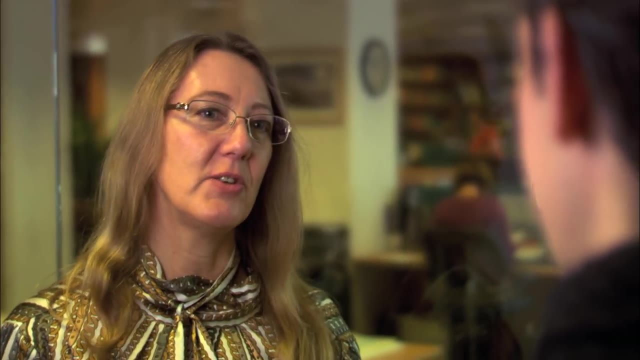 as well as a very strong scientific background, because they're going to go and have to deal with some very emotionally intense situations where people are quite upset about a situation. They're going to have to apply their science but also try and calm the situation and provide reassurance. 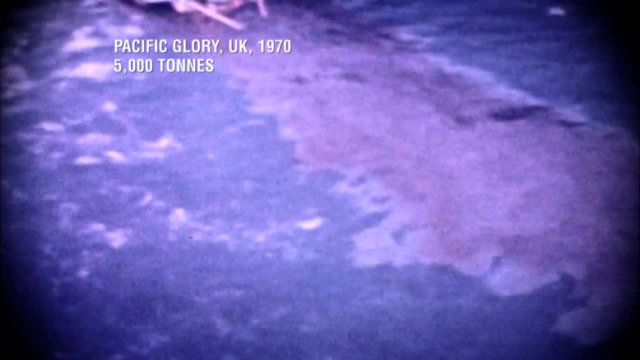 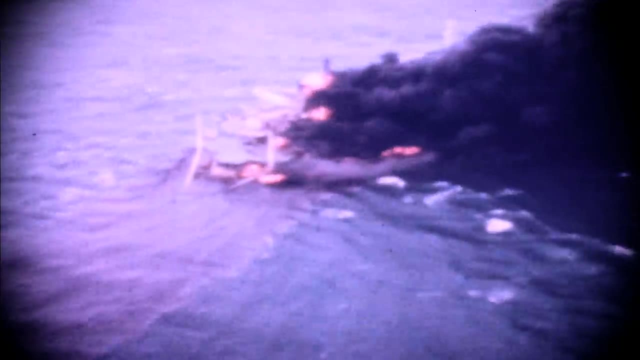 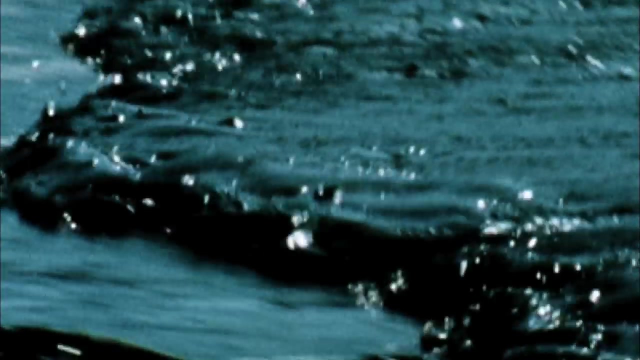 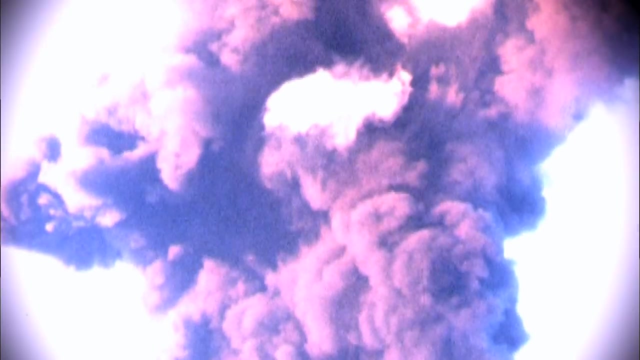 Just one of several oil tankers which have collided in the world's busy shipping lanes in recent years. ITOF's first decade in operation was a baptism of fire. The 1970s saw around 25 major tanker spills every year, With accidents releasing over 3 million tonnes of oil into the sea. 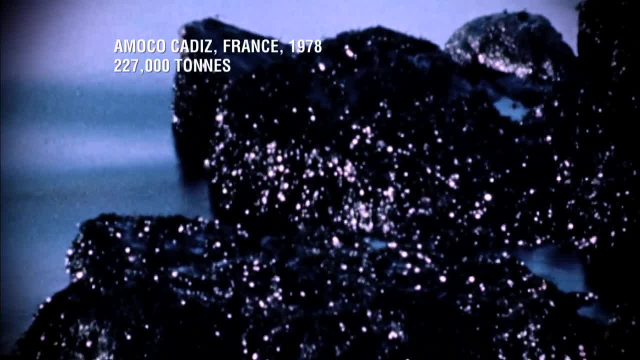 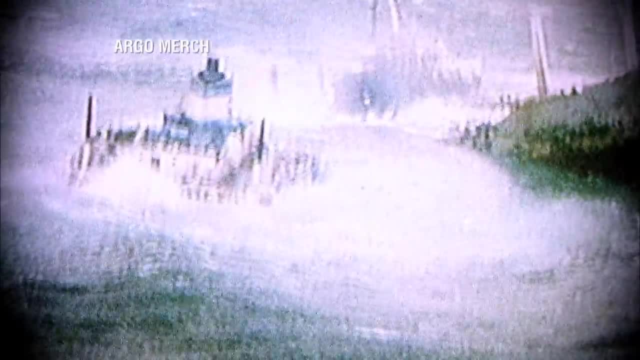 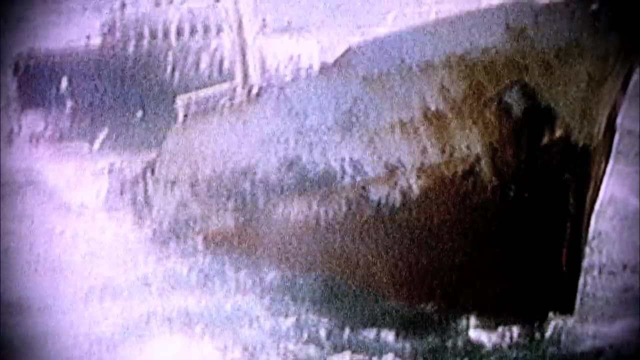 A black tide of oil from the wrecked tanker Amoco Cadiz, with a cargo of 220,000 tonnes of light Arabian crude. Within hours, the Liberian tanker had disgorged fully half its cargo of 6 million gallons of oil, according to Coast Guard estimates. 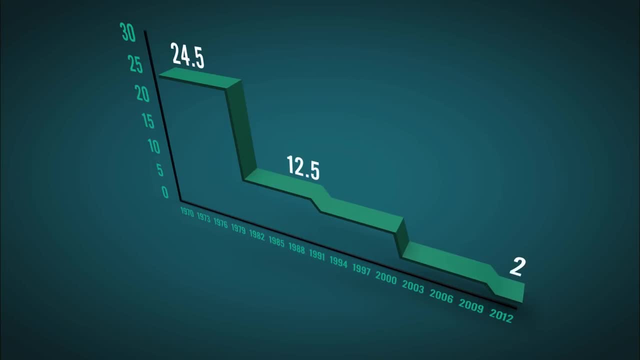 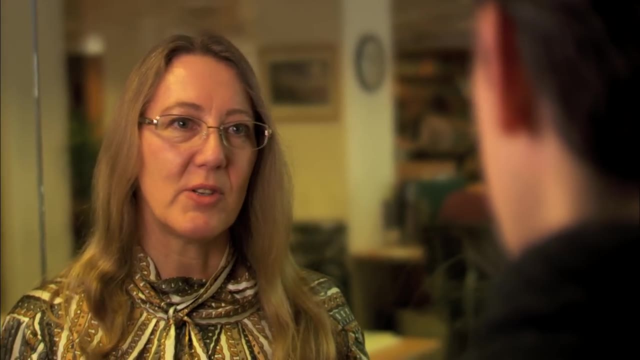 But since then the number of major spills per year, those over 700 tonnes- has dramatically declined. So back in the 1970s we were having 20, 25 large spills from tankers and the total amount of oil spilt was in the hundreds of thousands. Now, if you look at the last decade, two spills on average and we're probably talking just a few thousand. If you compare that to the quantity of oil that's actually carried by sea each year, it's a minuscule amount. So fewer spills and less total volume of oil spilt. 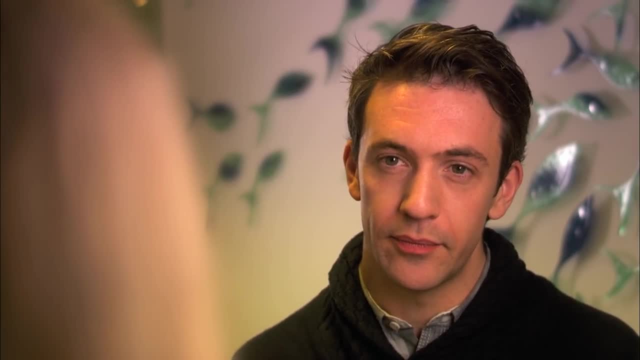 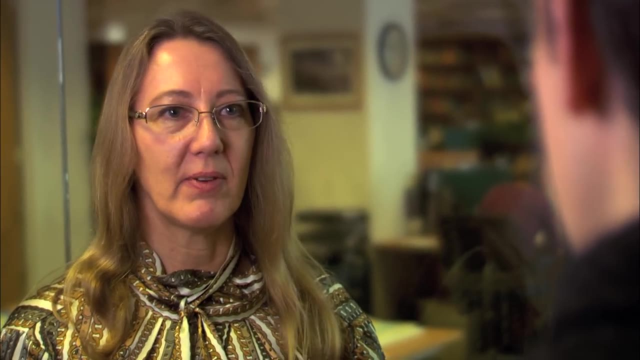 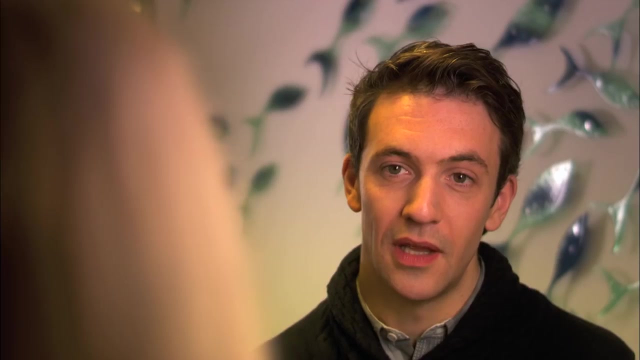 What would be a typical incident. today We're seeing more spills, probably smaller volume, from the fuel oil carried in ships like container ships and bulk carriers. So those now make up a larger proportion of the spills that we attend. And what challenges are posed by bunker oil or these heavier oils? Well, the type of oil that's spilt is much thicker. It's more persistent, So that oil can stay at sea for much longer. It doesn't break up like the lighter oils, And when it does come ashore it tends to smother things. 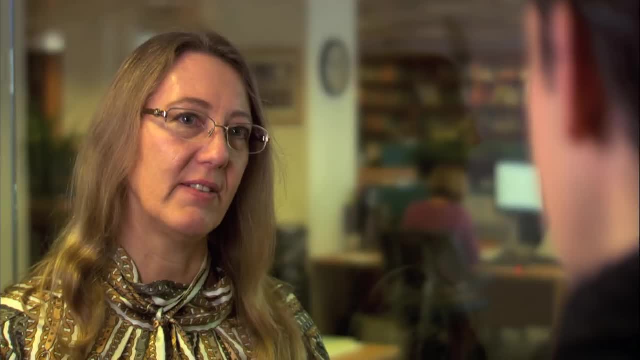 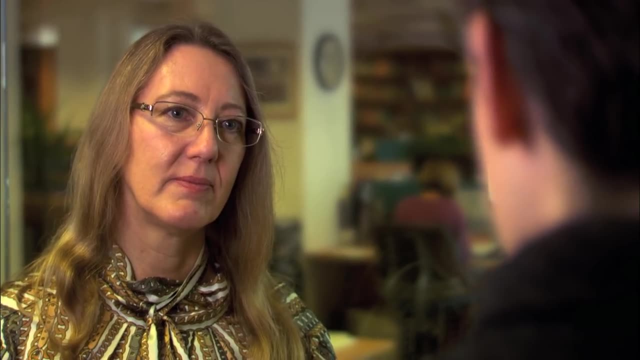 It can become very tarry and very difficult to clean, So it's more of a challenge when it comes to the cleanup. So even if you're dealing with a smaller volume of oil spilt, the technical challenges seem to be just as great. Absolutely yes. 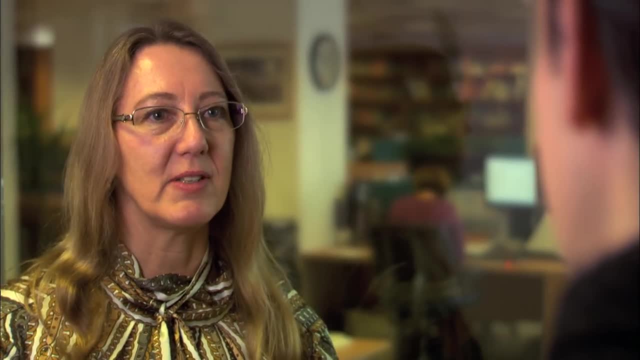 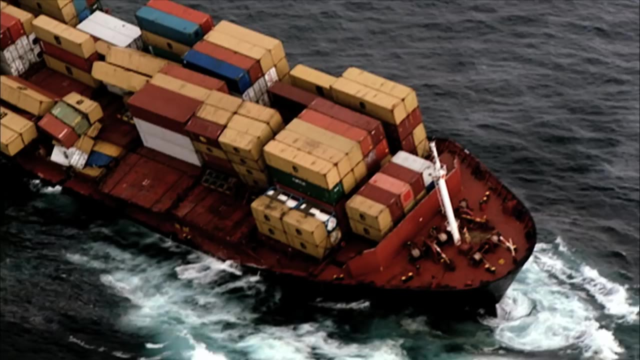 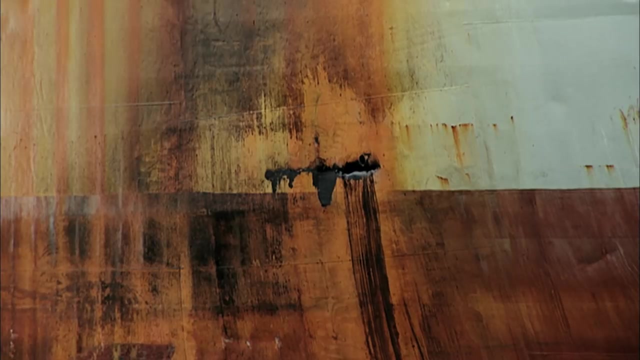 And the same emotional challenges. and actually even a small amount of oil through fish farms and seaweeds can cause a great deal of damage. As the challenge evolves, ITOF continues to advise on cleanup strategies and the effects of spills on the environment and people's livelihoods. 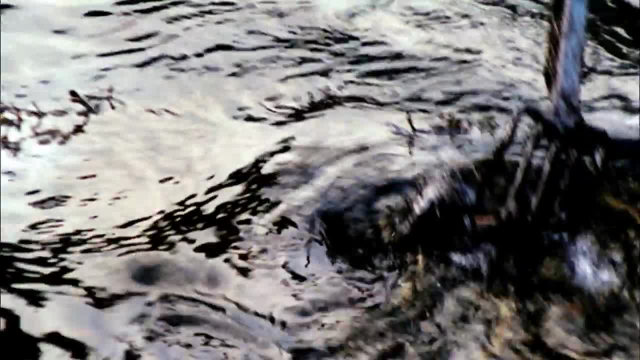 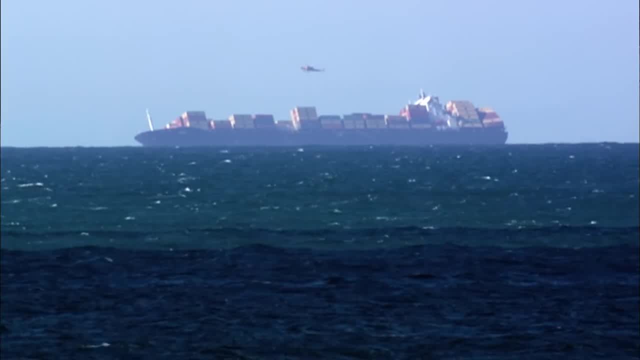 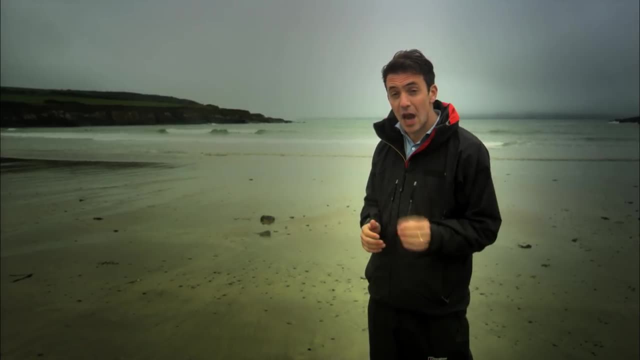 I want to find out how the lessons learned from previous spills can help us plan, respond and react to future incidents, Beginning with one crucial factor: Following any incident, it is really important to consider the type of oil that's been spilled. Responders need to establish quickly what they're up against. 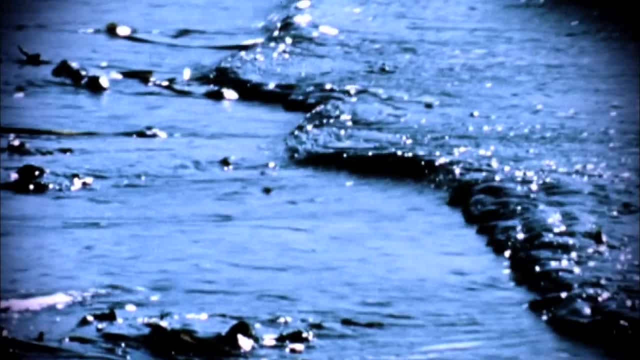 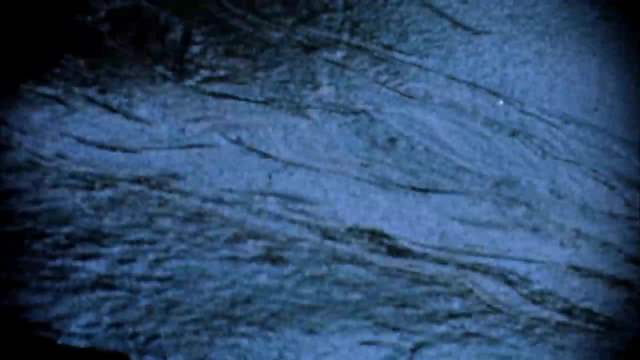 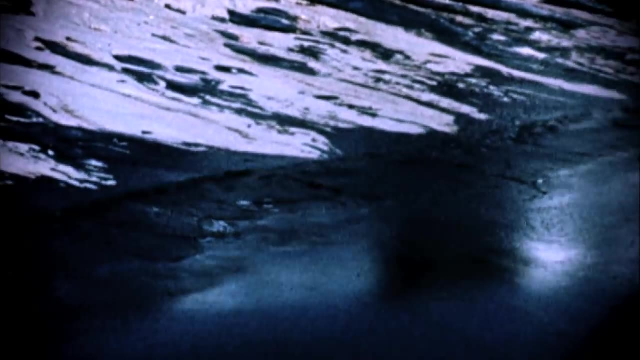 and tailor an appropriate response. When it comes to crude oil, the thing to remember is that it's a complex mixture containing many different hydrocarbons. Their physical properties can vary widely depending on where they're found and how they were formed. I've come to CEDRA in Brittany, a specialist research centre. 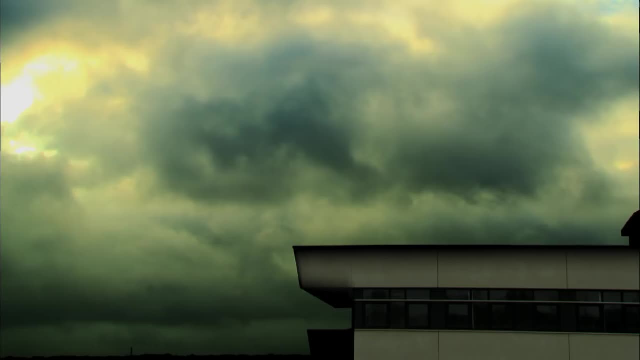 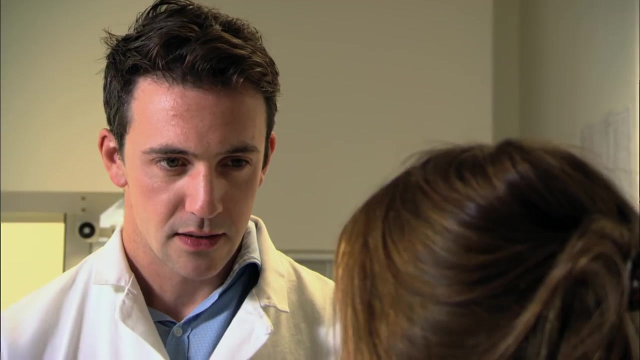 to find out how different oils behave in water. Annabel, sometimes when people in the public think of oil, they think of just one thing. but it's not quite as simple as that, is it? No, actually, oils are all mainly composed of hydrocarbons. 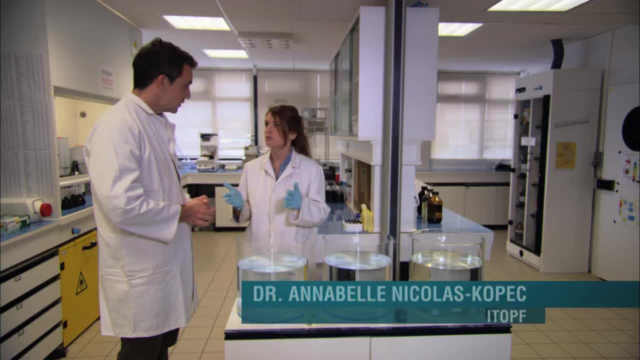 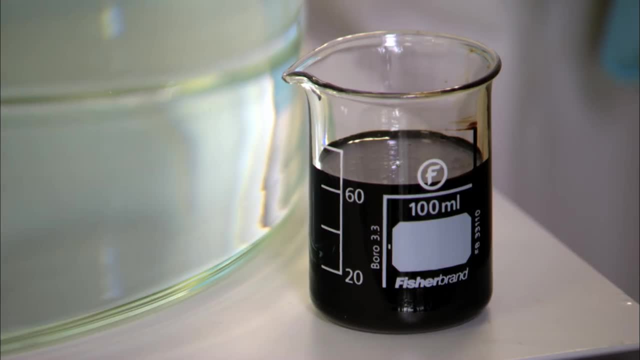 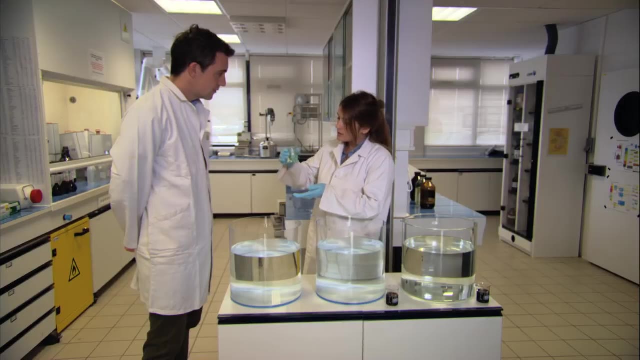 but actually their properties and composition can vary a lot, And here you have some sample of three different types of oils. We're going to see how these oils differ in their behaviour, starting with the lightest, a diesel. You can see it's a bit like water. 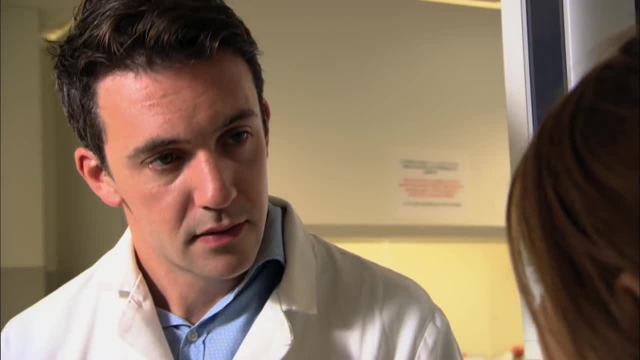 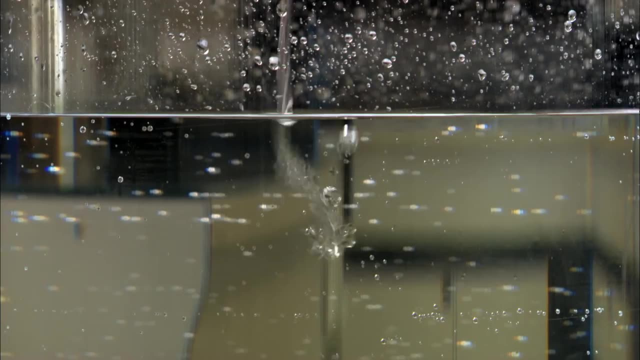 It's got a low viscosity, low density. If I pour it in the seawater it will spread really quickly. OK, and we can see that, can we? And we can see that The surface spread could be quite impressive, but the volume itself may be quite small. 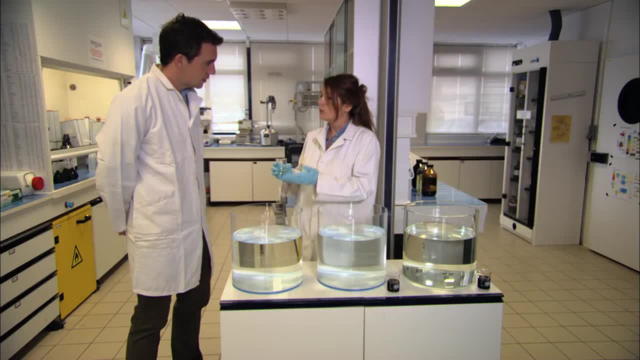 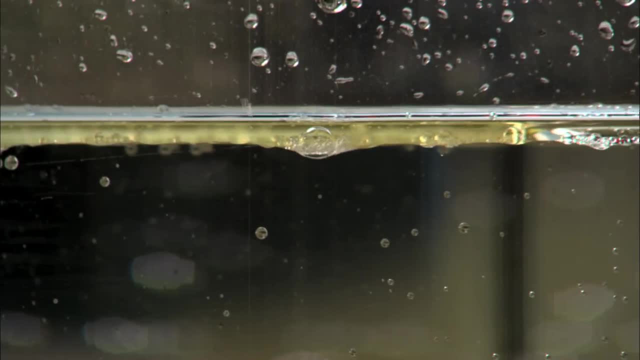 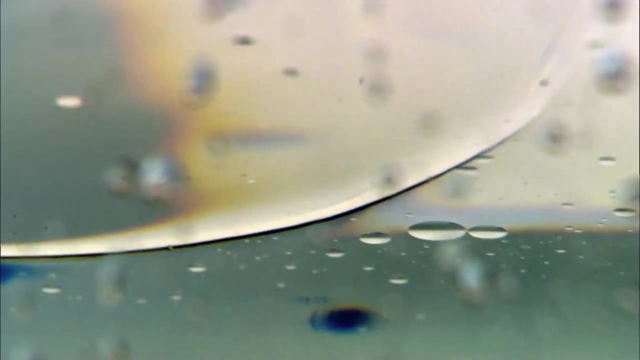 Just to give you an example, one litre of diesel actually can cover up to a football pitch surface. That's incredible. so a very, very thin sheen. Yes, As diesel is highly volatile, it will evaporate quickly into the atmosphere and won't persist long in the marine environment. 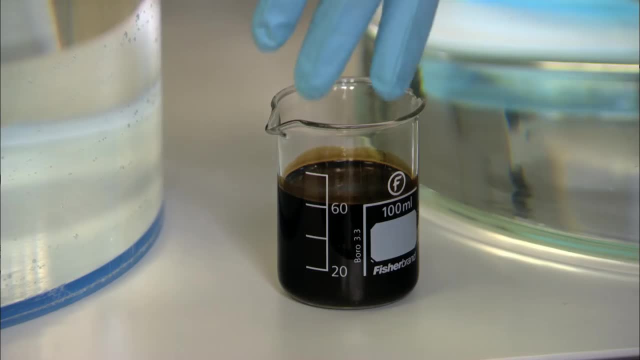 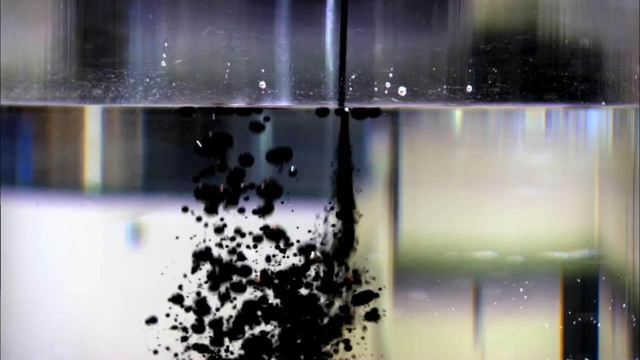 meaning a clean-up is rarely necessary. Next up a medium crude oil much more viscous than the diesel, and immediately you can see how it behaves differently. What's happening? you can see that it's spreading a bit, but not as much as the diesel oil earlier. 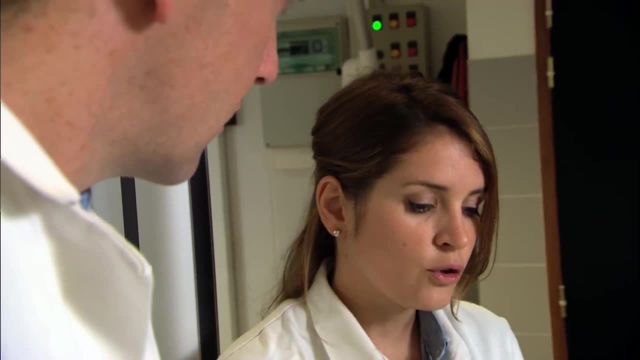 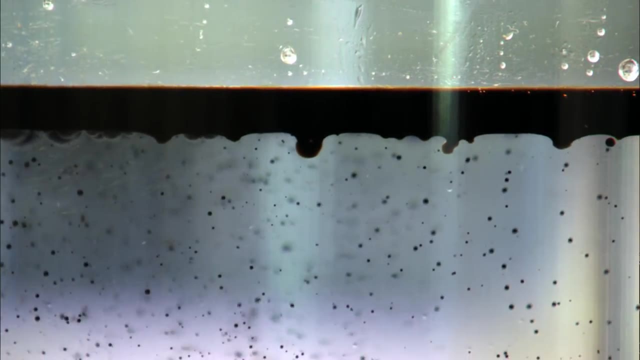 Around 20% to 40% of the crude is made of light products as well. So these 20% to 40% of the crude oil, 40% will naturally evaporate as well, reducing the volume of the crude but leaving some heavy compound in the marine environment. 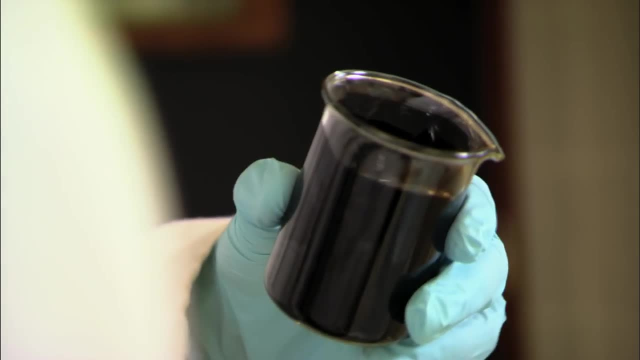 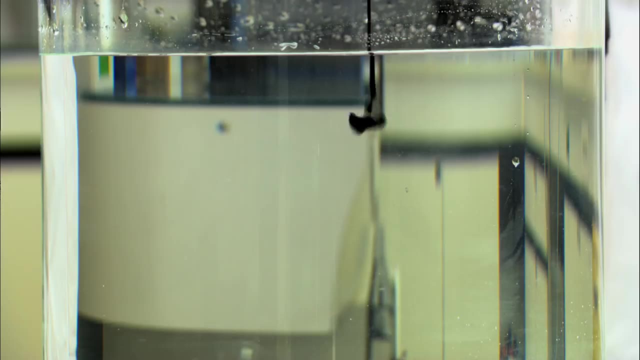 And finally, heavy fuel oil, or bunker oil. It's this that's used to power ships and it can represent a serious challenge for clean-up, Because it's very viscous, it won't disperse as much, it will not evaporate. 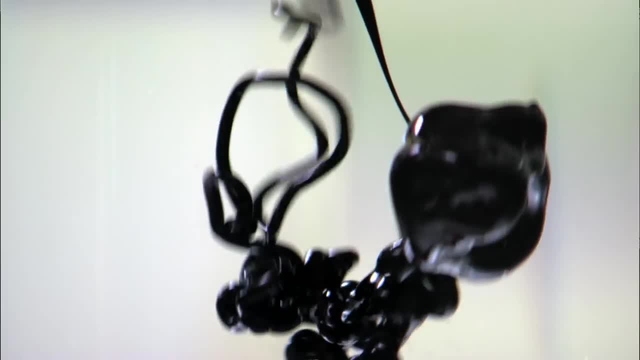 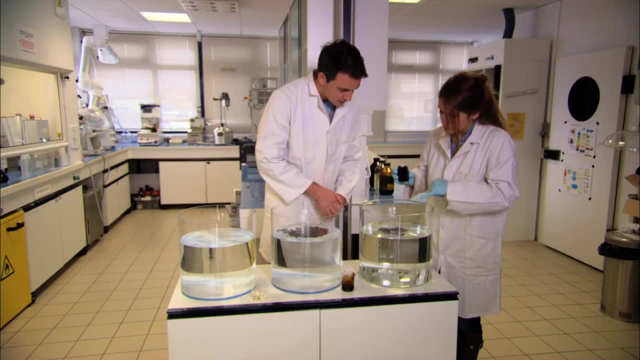 Usually you have less than 5% of light product. It really clings together, doesn't it? Exactly So. you see a tiny bit of the light compound evaporating, but almost not spreading. a tiny bit, but mainly the thick slick. 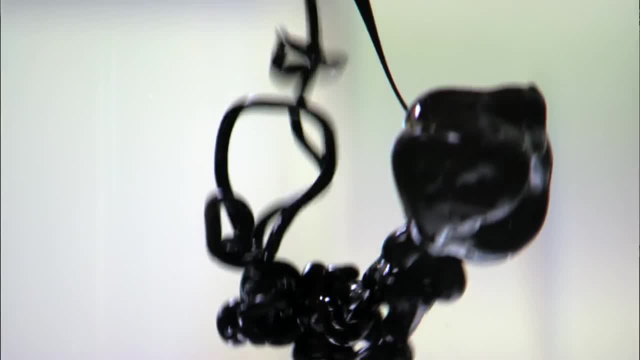 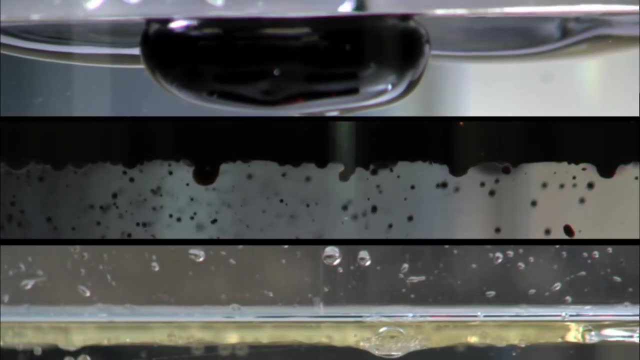 Fuel like this can persist as a semi-solid material at sea for a long time. It's clearly a completely different proposition to the crude and the diesel, and it's crucial for responders to understand these differences in order to apply the right clean-up techniques. 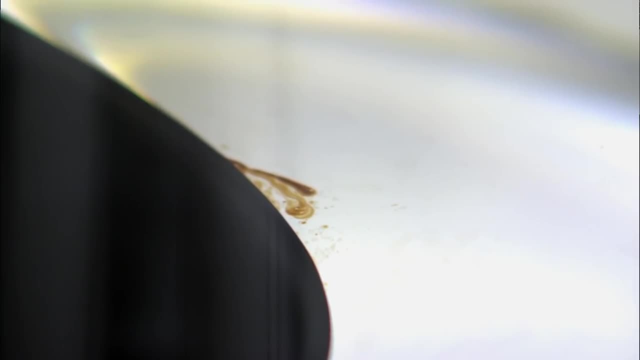 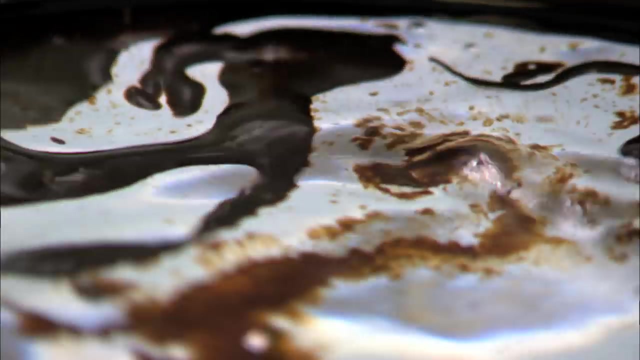 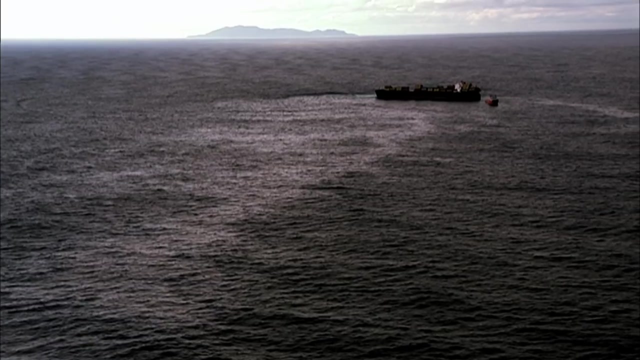 But understanding the type of oil is only one part of the jigsaw. You've also got to take into account how it will behave at sea. At sea, most oil will spread rapidly, potentially covering hundreds of kilometres in just a few days, As it's subjected to waves and wind. 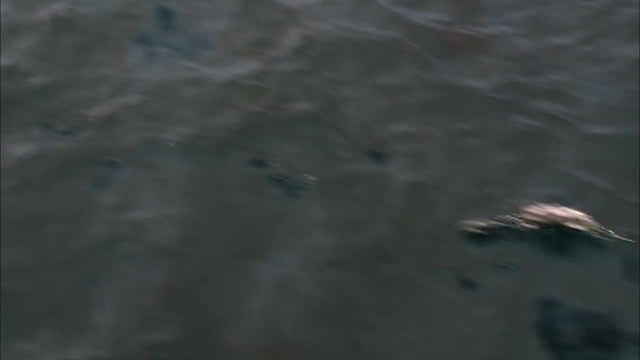 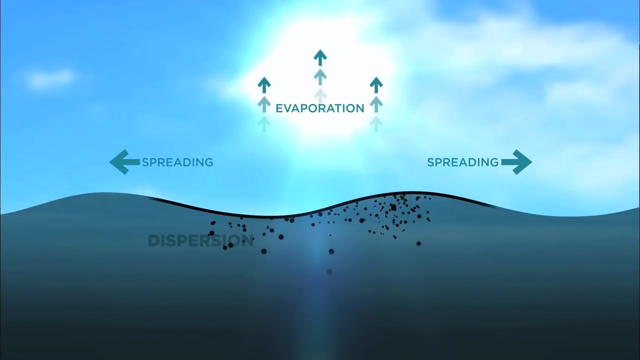 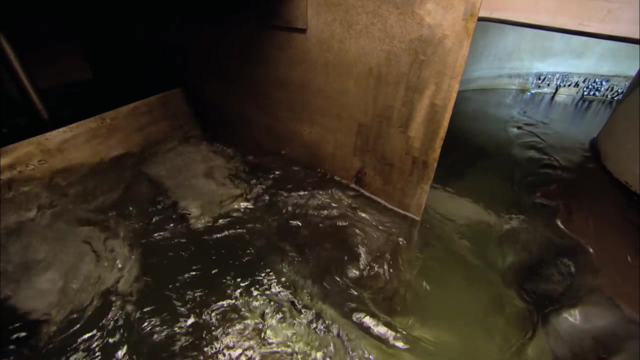 it'll undergo a range of physical and chemical changes known as weathering. Understanding weathering and how the individual processes affect the behaviour of oil is the cornerstone of oil spill response. so I want to get to grips with the basics. This piece of equipment is capable of simulating these processes. 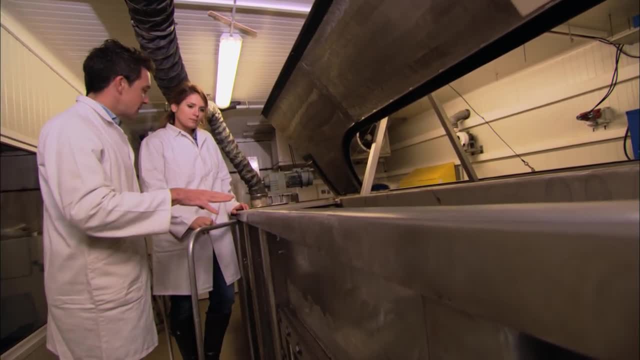 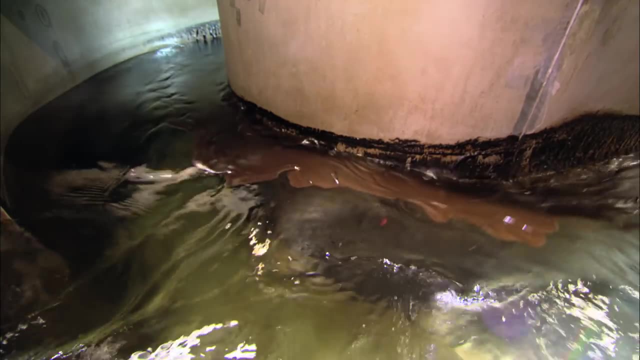 Now, beakers in a laboratory are one thing, but this is really stepping up the scale. What's going on here? Well, we are here in the political room And you can see here, on a much smaller scale, what will happen at sea. 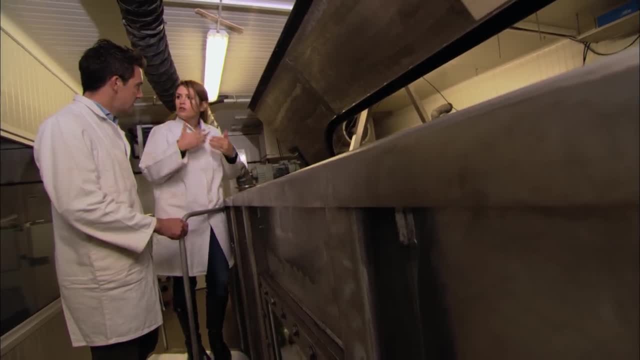 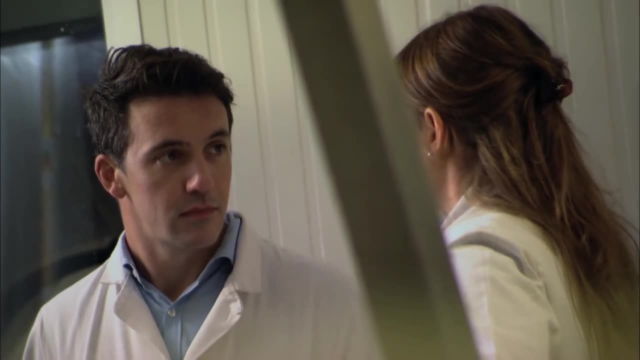 You have the wave, you've got the current, the turbulence, and you have the wind, And so it will alter the composition of the oil. Two days ago, this medium crude oil was placed in the polydrome in order that the effects of weathering could be observed. 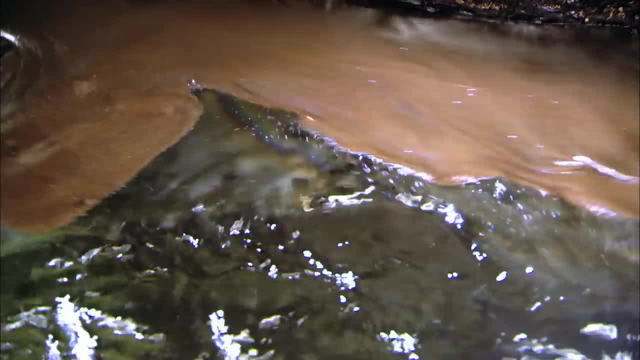 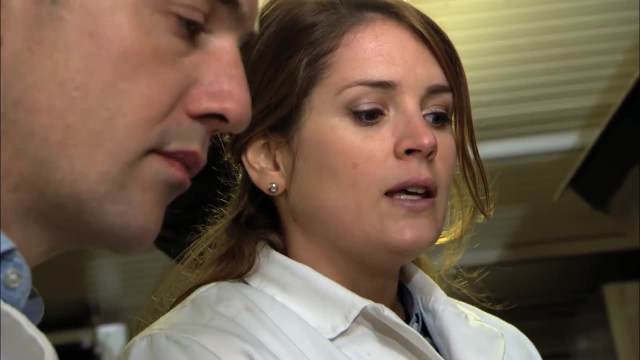 You can see already it's very different to the one we had in the beaker. You can see here it's much more viscous, The crude oil. it's much more viscous. The colour changes The reason is because the light compounds already evaporate. 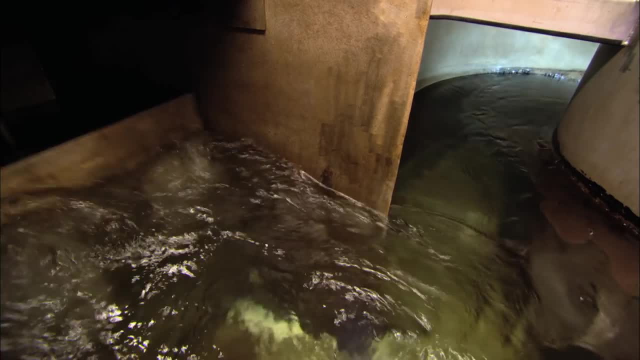 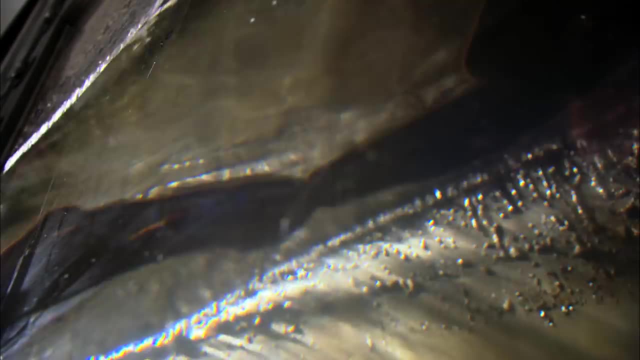 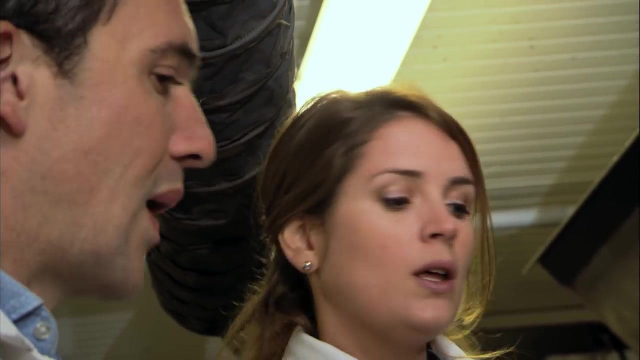 and you have different phenomena. that started already. The one that has the most action is what we call a watering oil emulsion, when you have droplets of water that are mixed in the oil And that will increase the volume, sometimes up to five times. 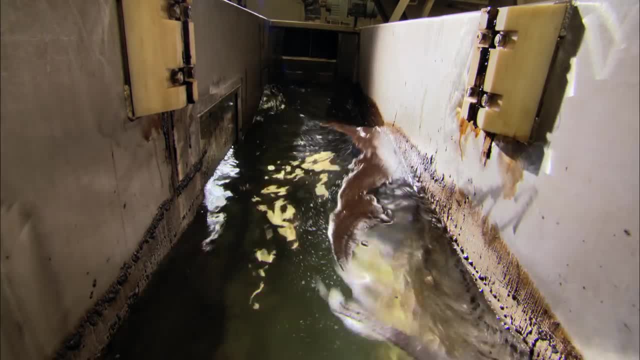 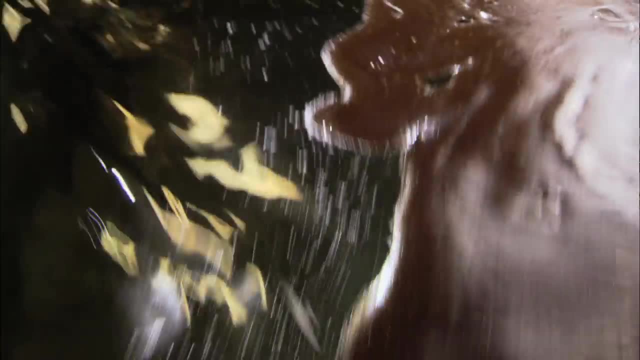 Wow, Yeah, And it will give this consistency. It's a bit what we call sometimes a chocolate mousse in the sling. So the volume of this oil has changed even in two days, because the water droplets in the oil are making it spread out, increasing the volume. 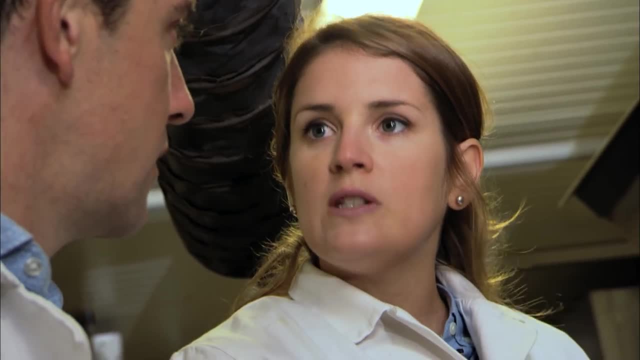 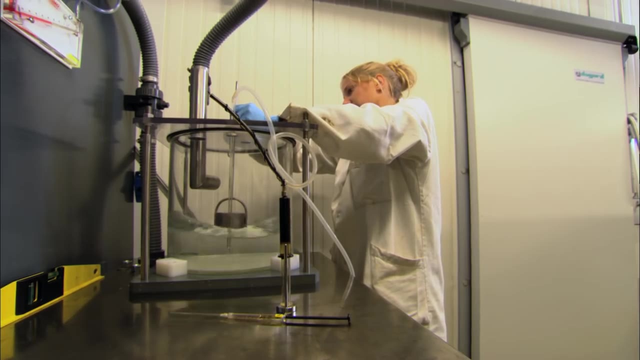 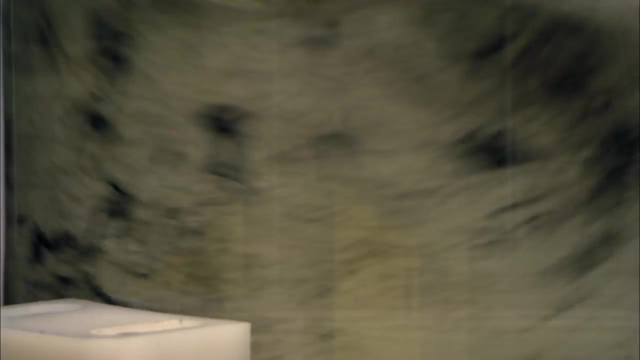 Exactly, And it's going to be much more difficult to deal to respond to this type of oil than to fresh oil. Oil will also disperse naturally into the water column, as this experiment demonstrates. Larger droplets resurface, but smaller droplets are kept under the surface by the turbulence. 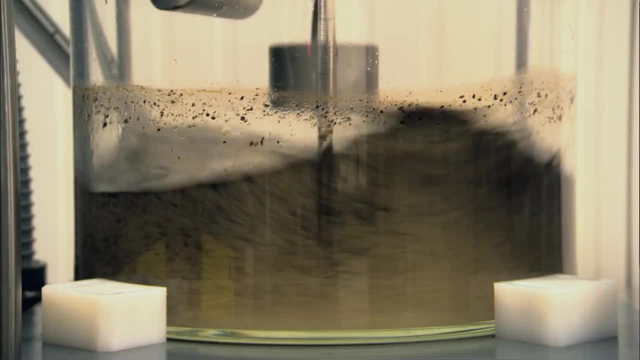 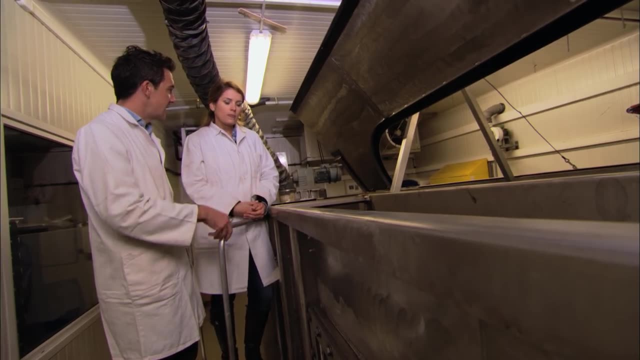 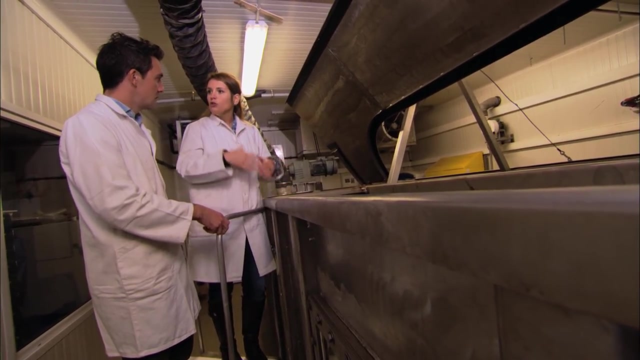 They're diluted and eventually broken down. Natural dispersion is a key process for responders to understand Just how important are experiments like this for understanding the behaviour of oil. It is really important to understand how oil behaves so you can be prepared in case of a spill. 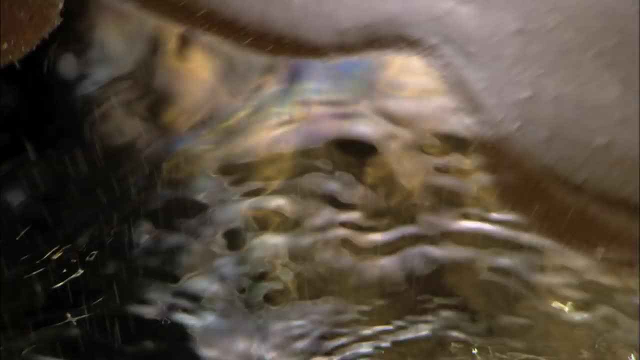 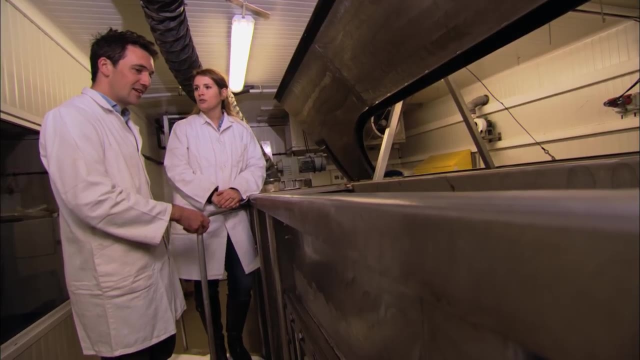 if a spill occurs, to have the proper equipment to respond to a particular type of oil. So there's a lot of variables here, A lot of variables. So this type of apparatus is very useful. Processes such as spreading, evaporation, emulsification. 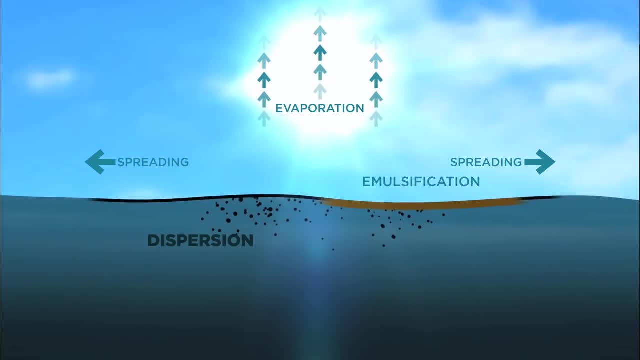 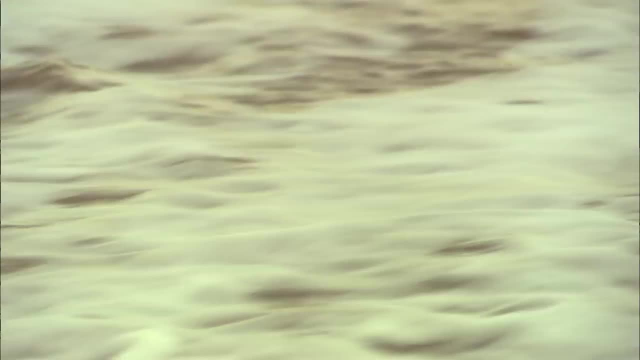 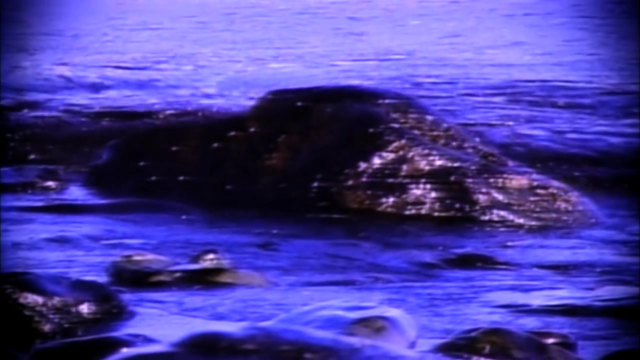 and dispersion interplay differently with different oils. Understanding this is critical to planning an effective response to spills. Take a look at this: In 1989, the Exxon Valdez runs aground in Prince William Sound, Alaska. A large proportion of the crude oil comes ashore. 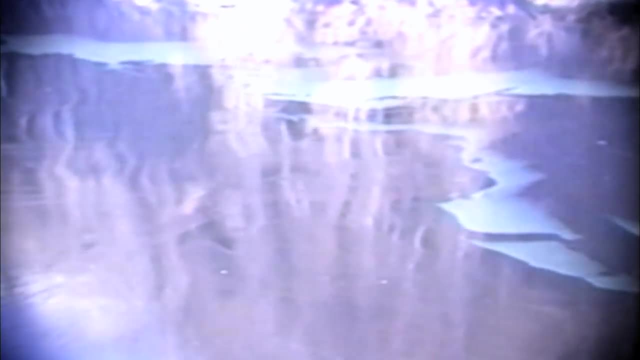 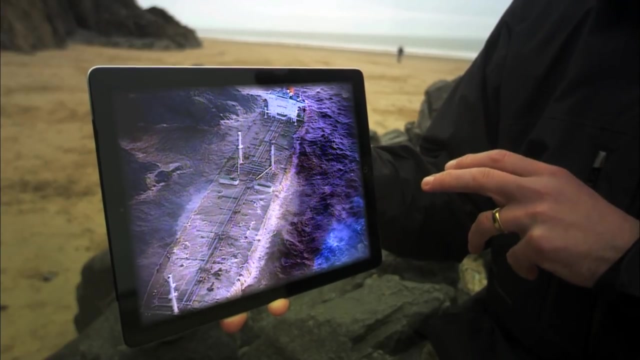 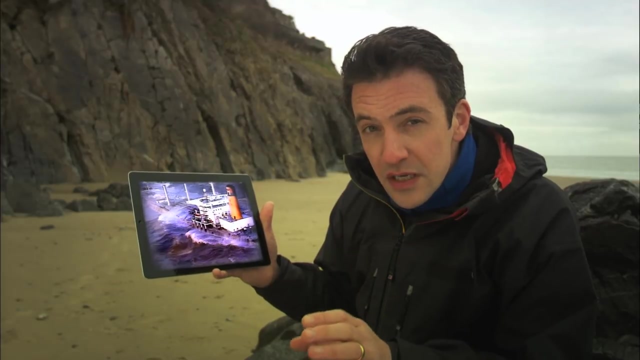 and the environmental impact in particular is severe. But now look at this: Four years later, the Brer is blown onto rocks off the Shetland Islands. More than 85,000 tonnes of oil spill into the sea. That's twice as much as the Exxon Valdez. 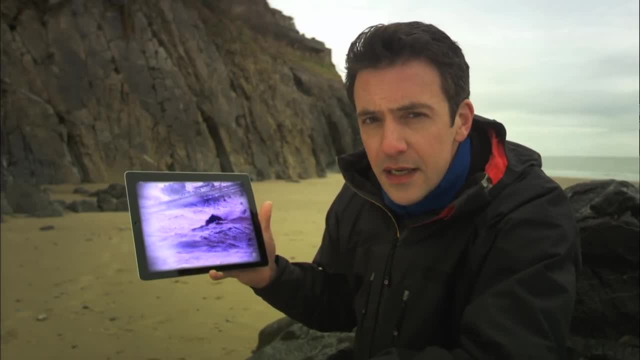 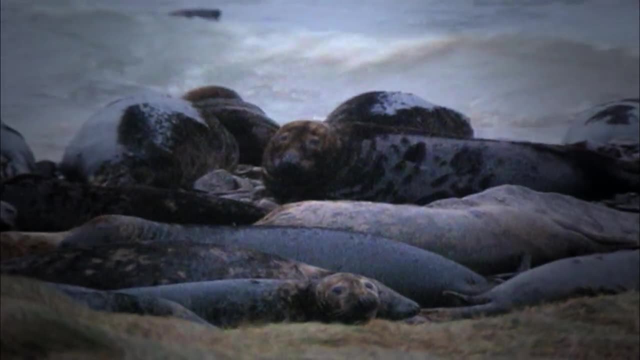 So you'd think the impact would be twice as great. The Shetlands were braced for catastrophe, but it never arrived. In fact, the economic and environmental impact was relatively small scale and there was little need for it. So what's the need for a spill response operation? 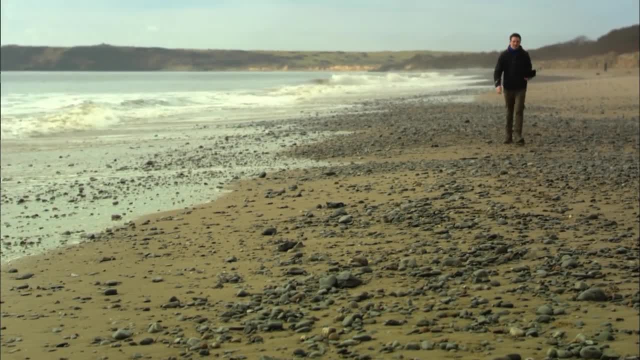 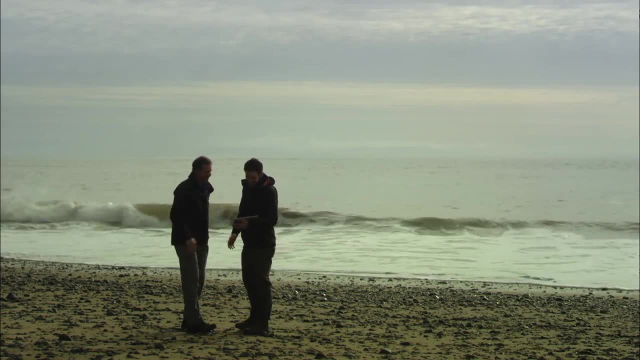 The answer to why rests in understanding the types of oil spilled and how they interacted with the conditions. Dr Tim Linnell from ITOF attended the incident. Tim, this is a huge spill and yet the shoreline isn't too badly affected. 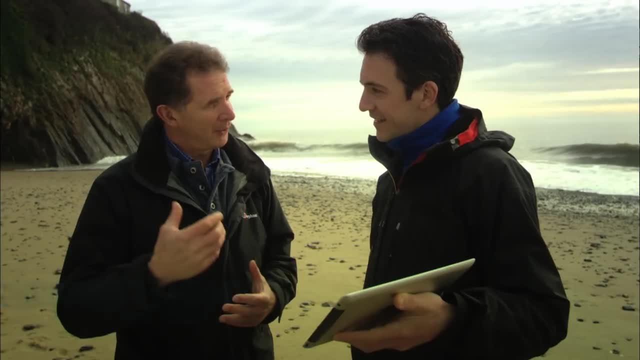 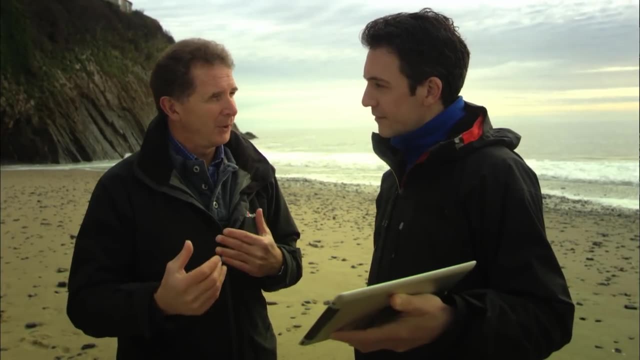 So what happened? Well, it was very much around the fact that the oil that was spilled was a light crude oil called gulfax And that was very low viscosity, And so it actually didn't form the sort of water and oil emulsions 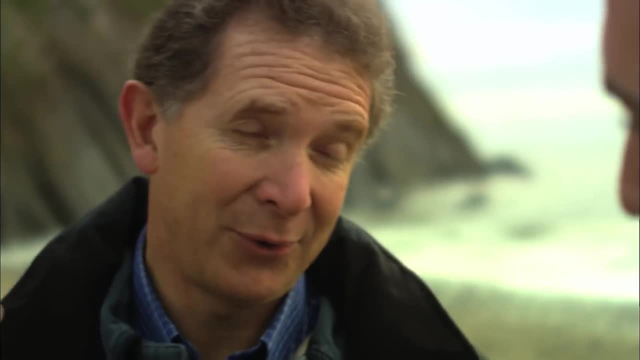 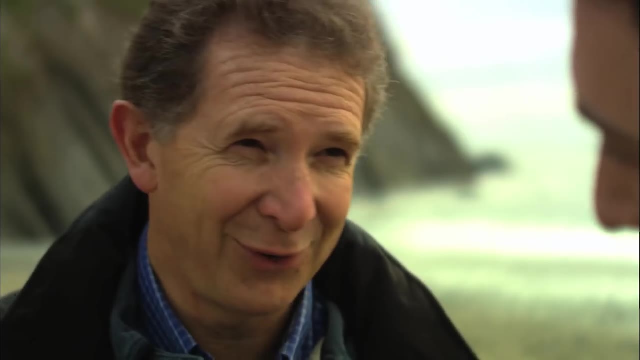 which can make manuals very persistent on the sea surface. And of course then, added to that, you can see the crashing waves there And you know the force of the winds. there was forced 11 to 12 winds, gusting 13,, 14.. 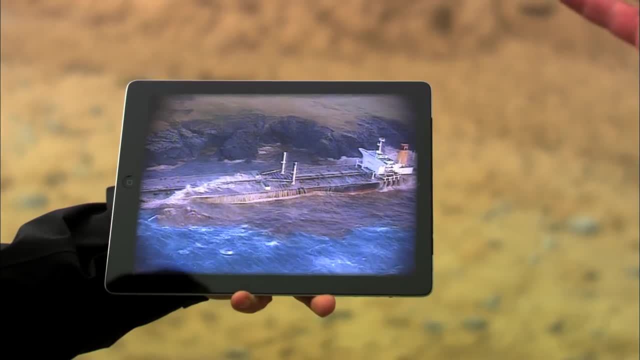 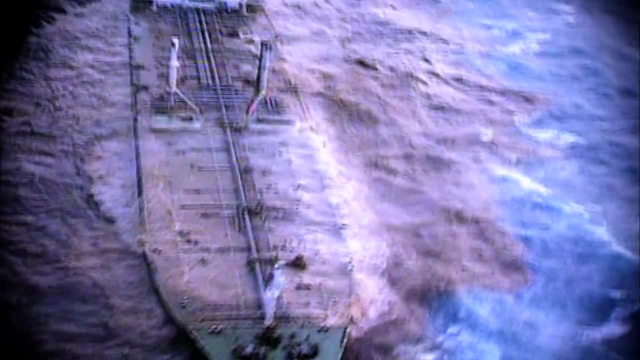 So it was pretty wild out there. You can see the waves actually breaking that slick up and dispersing it into the water column And in fact, if you look around the Brer itself, the vessel itself, you can see that kind of coffee-coloured plume to it. 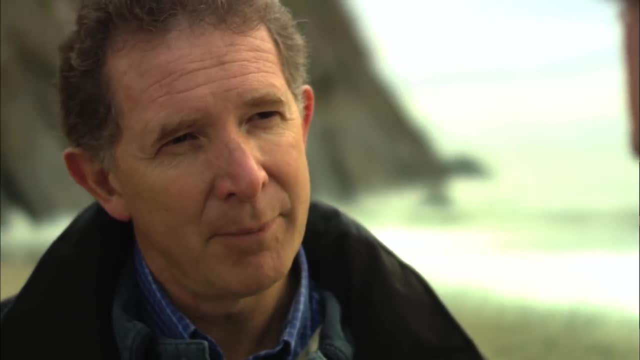 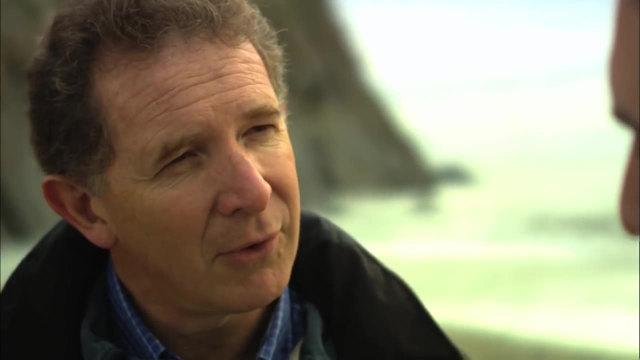 Yeah, And that's actually the visual evidence to show that the oil is being broken up into these really small oil droplets, So something like really tiny ones about 70 microns in diameter, and then just diluted over time. Wow, And you can, I mean, see the energy of those waves? 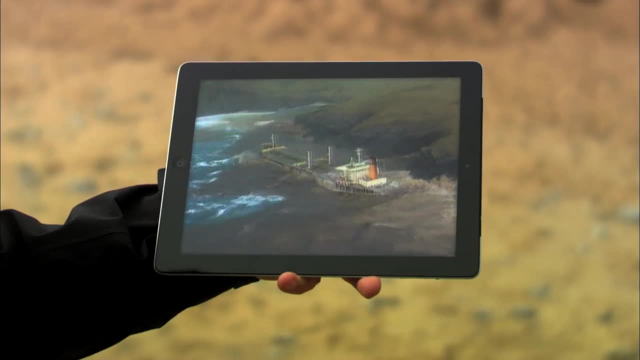 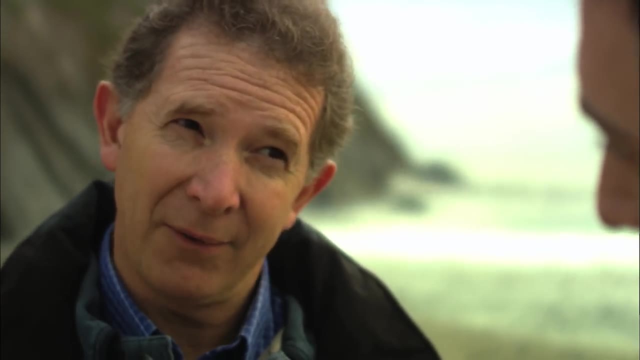 How long did those conditions carry on for? Well, that was the thing. Those conditions carried on for 12 days or more, So that kind of continued to break the oil up and spread it over a very large area. The heavy seas also had sort of. 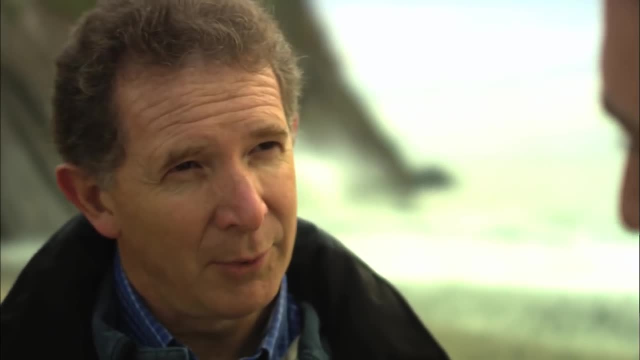 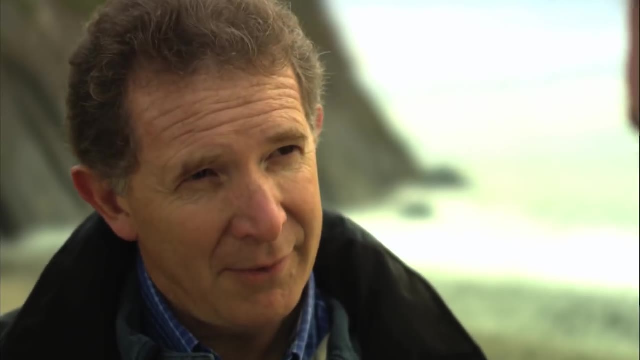 very fine suspended sediments in the water. The oil interacted with those and again really helped to spread it over a very large area. interacted and then the naturally occurring marine bacteria out there helped to degrade it over time. And what that meant was there really wasn't. 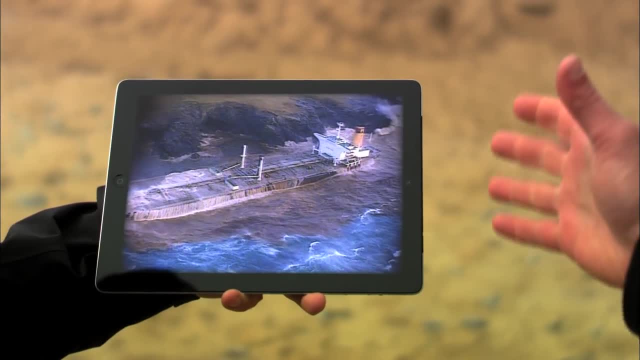 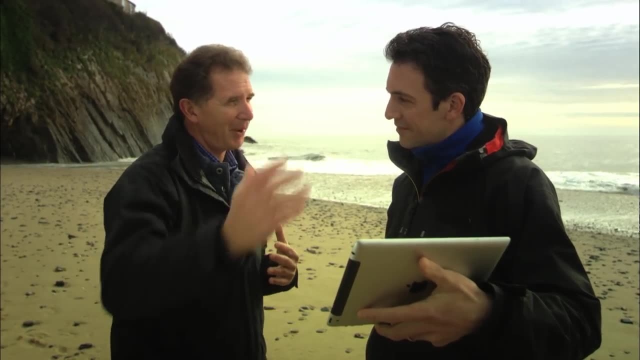 a surface slick And you can see in the area around the vessel there on the beaches. I was there first-hand and you can see these head highways crashing in, coming up the beach but then washing back out again. So the black waves came in. 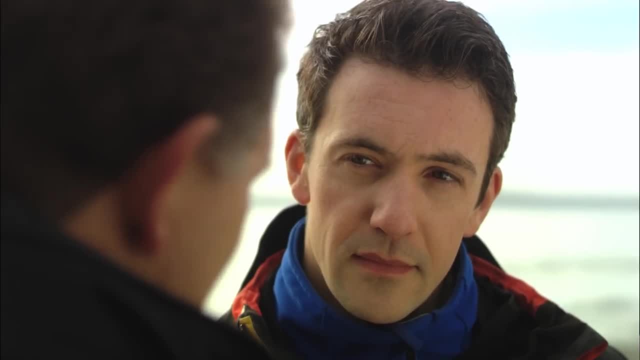 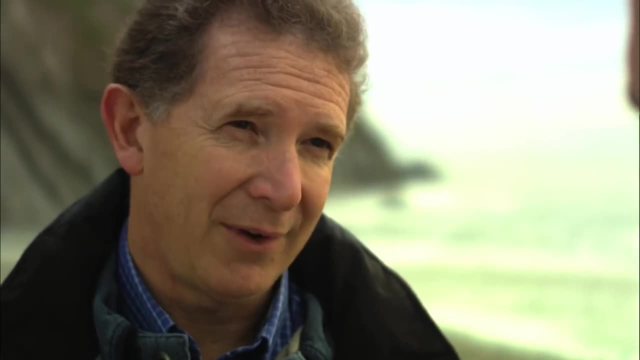 but they came out without leaving that sort of characteristic span line And what that meant was that, you know, compared to the Exxon Valdez, you had twice the volume of oil at the Brea, but actually the sort of environmental impact was pretty minimal. 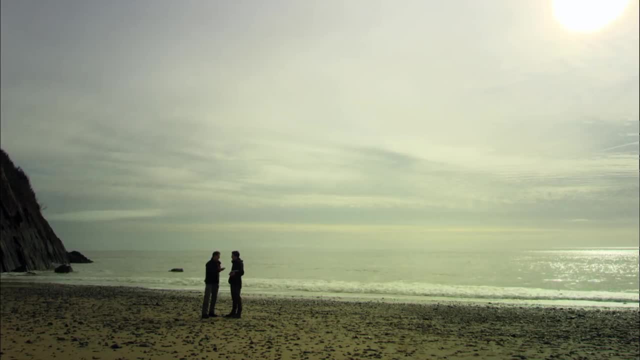 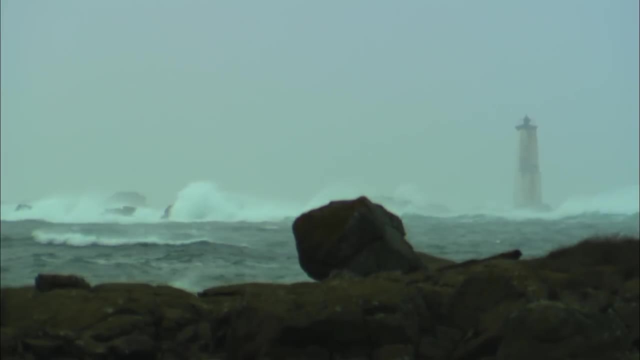 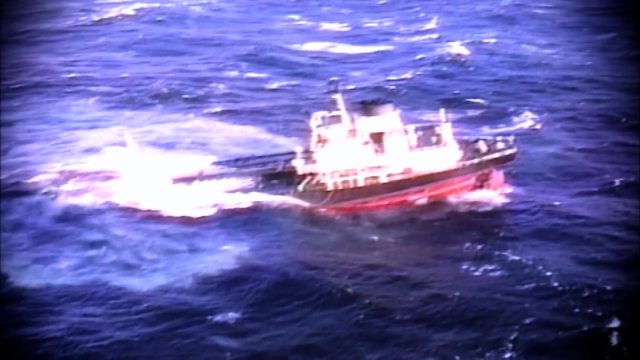 And that's because the fate of the oil was determined by the process of evaporation and natural dispersion. But strong seas aren't always good news. Depending on the oil type, the churning of the waves can sometimes make the problem much worse. For example- look at this- the Erika in 1999.. 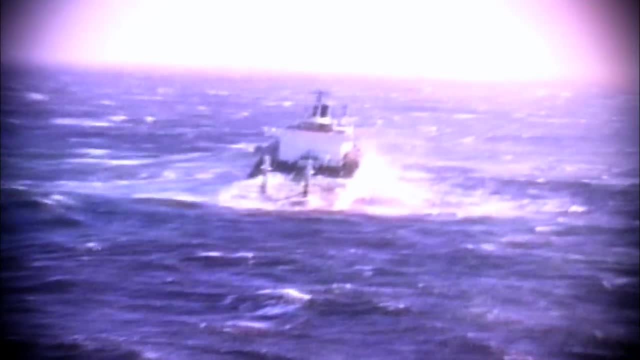 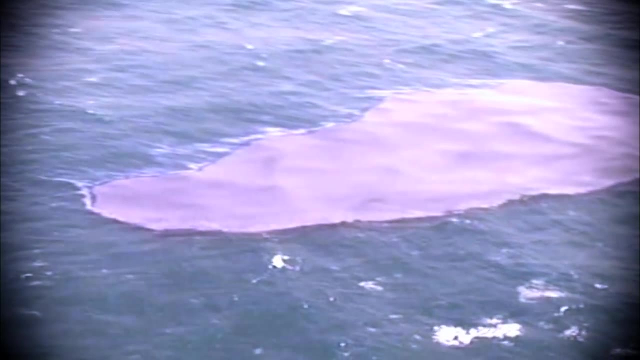 Similar sea conditions but, crucially, a different oil type. On this occasion, it was a heavy fuel oil that was spilled. As we've seen, it's a completely different prospect, As the Maltese tanker sank off the French coast, the churning action of the waves, 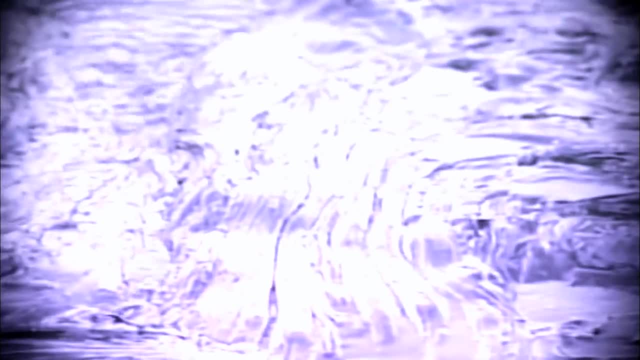 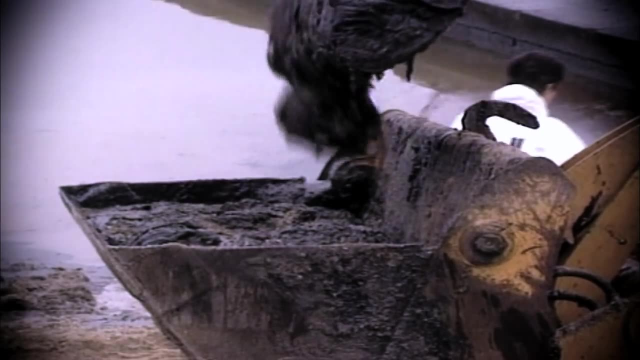 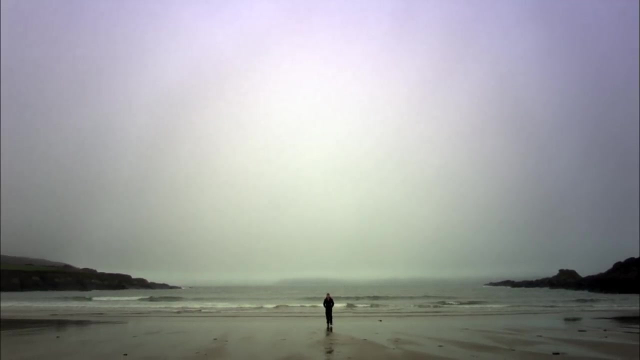 captured droplets of seawater in the slick, creating a viscous emulsion, And here's the result: a shoreline that was heavily contaminated, and a large-scale clean-up operation followed. So far, we've seen how processes such as spreading, dispersion, evaporation and emulsification 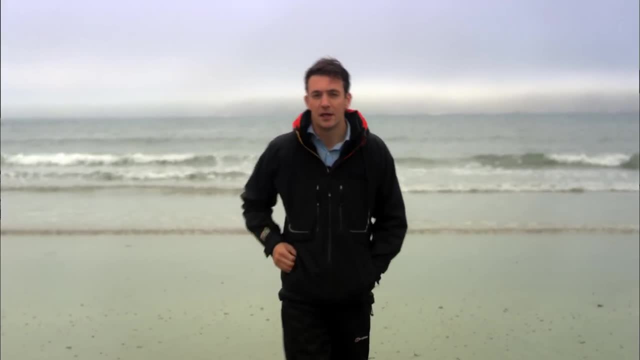 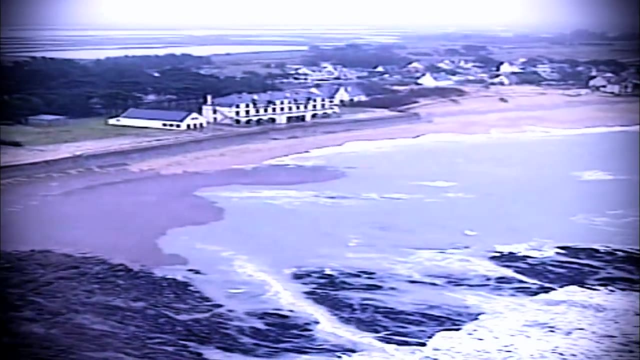 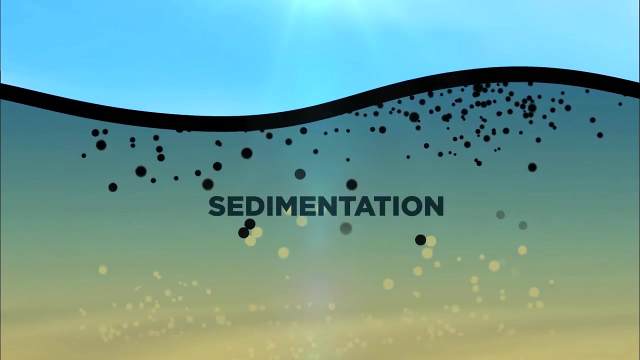 act on the oil immediately after a spill, But there are other processes to consider which take a bit longer. A less frequent process that can happen in shallow water is sedimentation. This is when sediment stirred up into the water column by intense wave action. 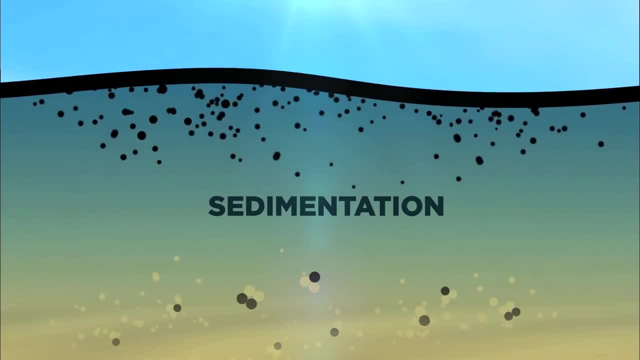 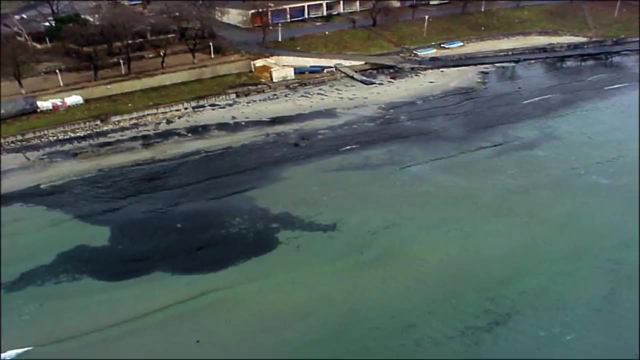 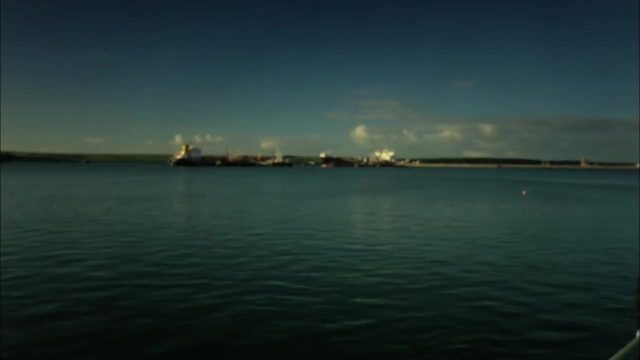 mixes with dispersed oil droplets and then slowly sinks to the seabed. When floating patches of heavy oil pick up suspended sediment, they can also sink to form dense tar mats, presenting a challenge for the response. There's actually another process to be aware of. 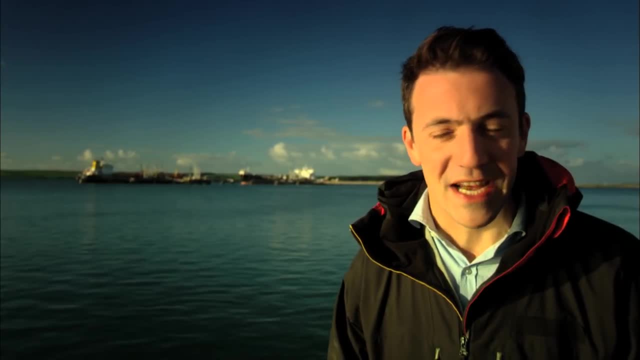 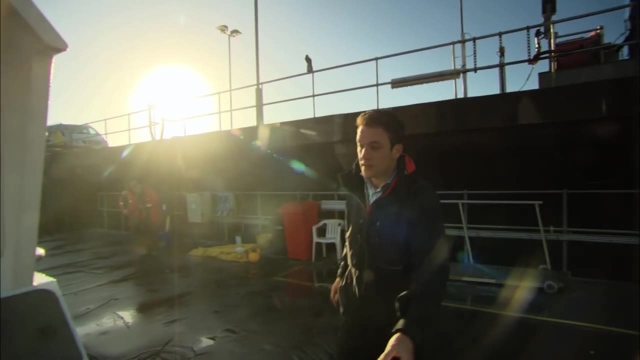 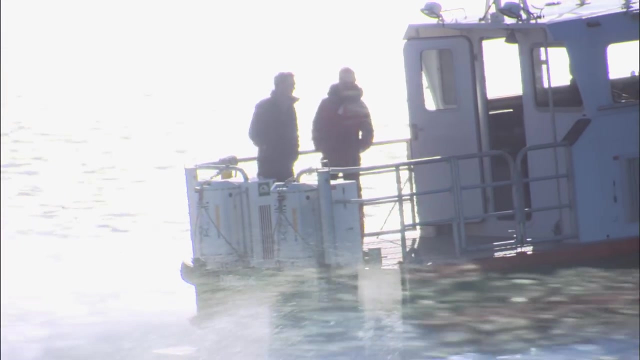 It may be slow, but it's one of the main mechanisms for getting rid of the last traces of oil from the marine environment. To find out more, I've come to Milford Haven to meet marine ecologist John Moore. He's attended spills all over the world. 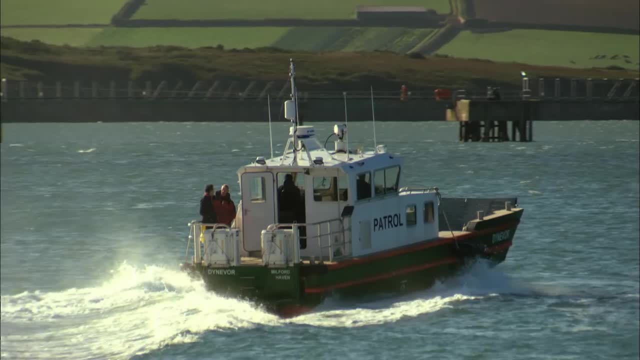 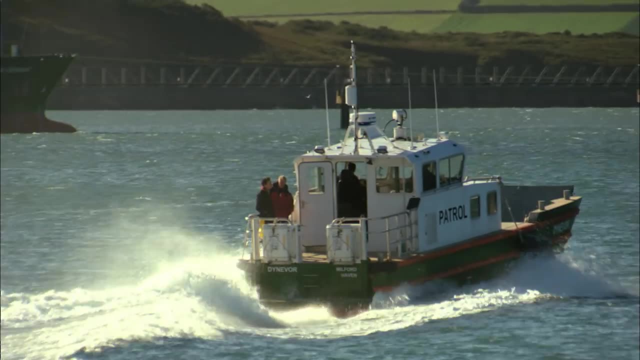 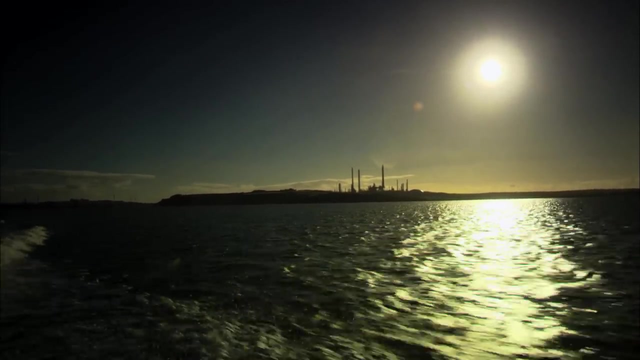 and has spent many years studying their impact on marine organisms and communities. He's offered to explain how oil in the water is by no means a modern phenomenon and how nature has equipped itself with a solution. Oil is a natural material. It came from life eons ago underground. 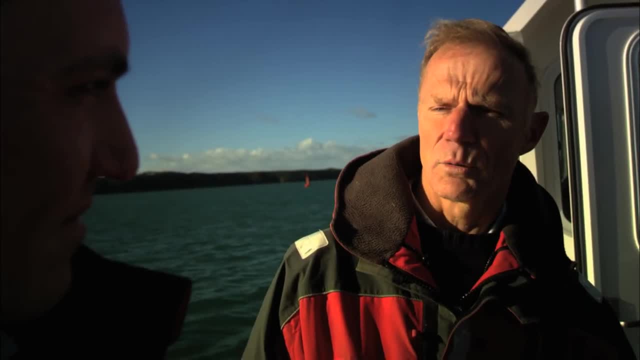 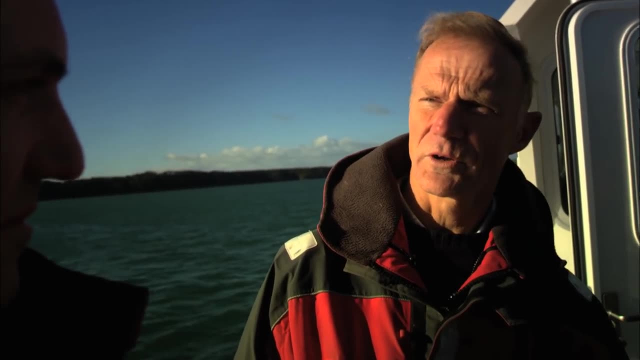 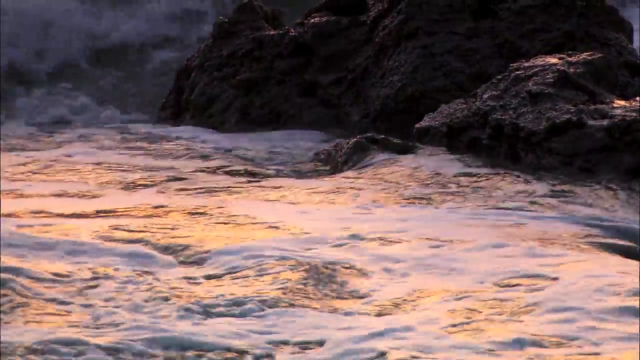 and in many places it does still seep out. We're using it and life has adapted to use it. Over millions of years, life has evolved to use it as a foodstuff. The sea is teeming with microscopic organisms, some of which are able to break down oil. 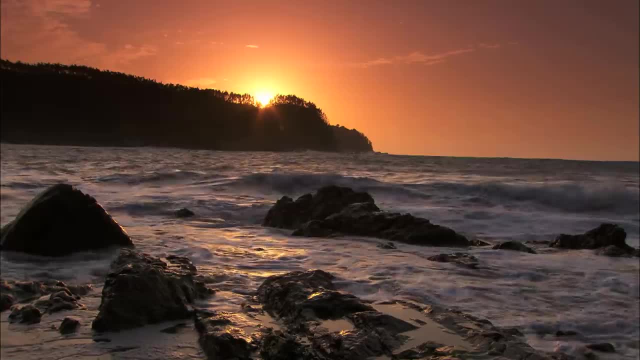 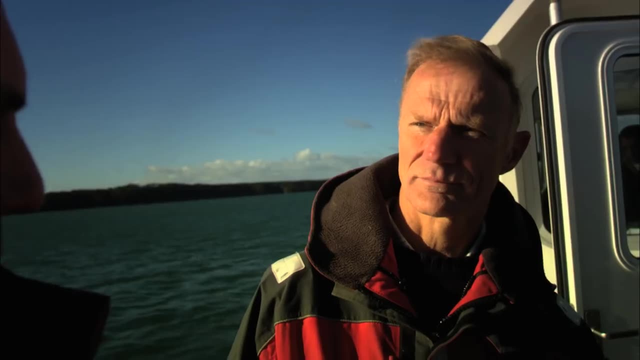 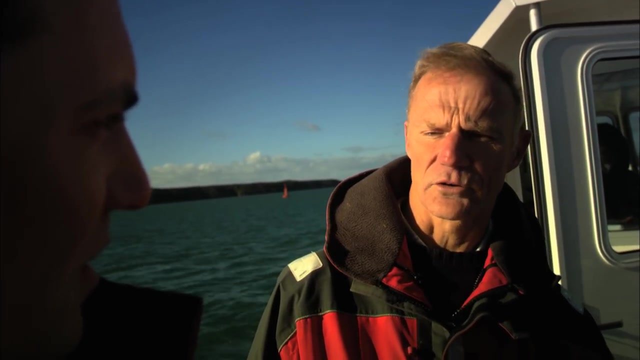 into water-soluble compounds. It's a process known as biodegradation, And so when a spill occurs, what happens? Do these bacteria get to work immediately? Bacteria that are present in the water in large amounts are immediately attracted to it. 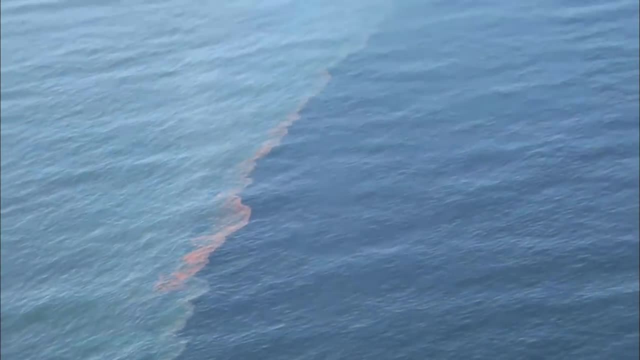 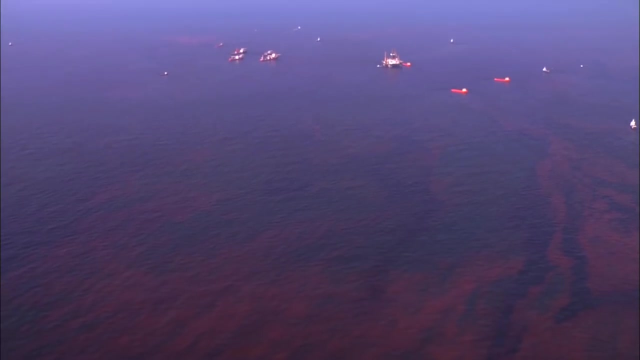 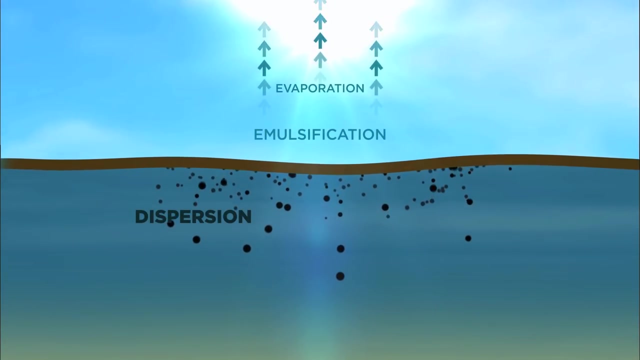 They will attach to the surface of the oil and start to break it down And obviously the larger the surface area there is of oil, the more bacteria can get onto it, multiplying rapidly and breaking it down more rapidly. If the oil is broken up into small droplets, 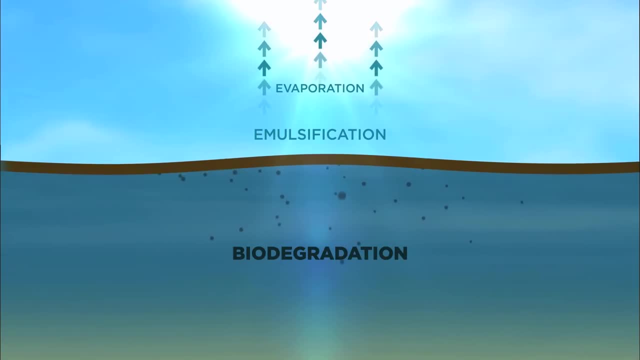 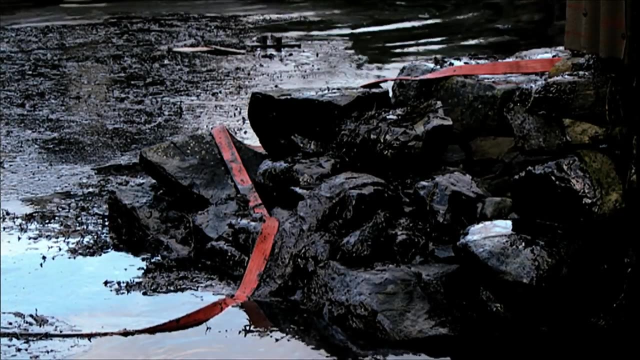 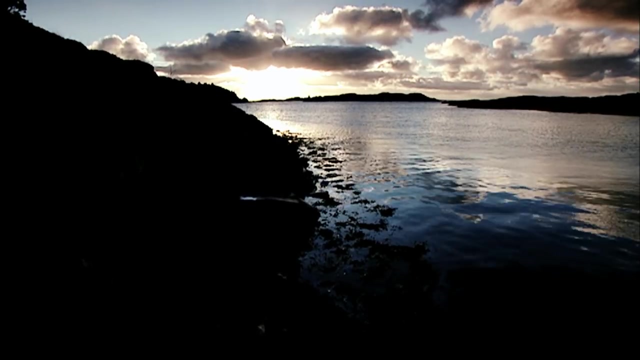 into the water column through natural or chemical dispersion. this increases its surface area and accelerates biodegradation. By contrast, it's much slower if the oil is lying in thick layers on shorelines or if it gets mixed up with sediment on the seabed. 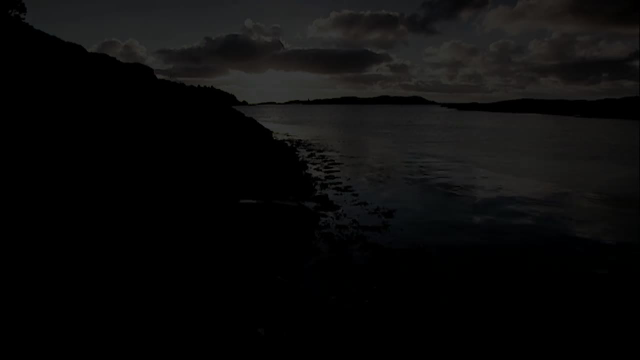 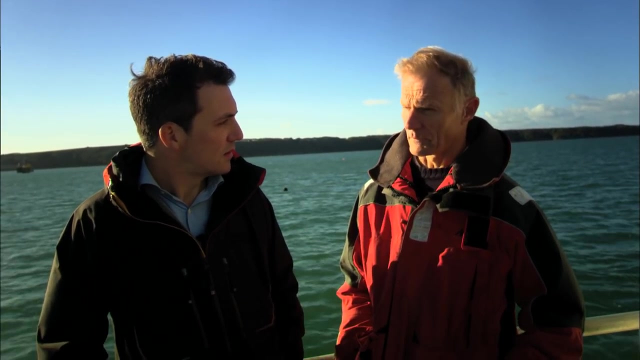 So this isn't a substitute for removing bulk oil, but this is a process that sort of cleans up the rest of it once a lot of the response has happened. Well, all the oil that gets removed and remains in the marine environment that we haven't taken out of the environment. 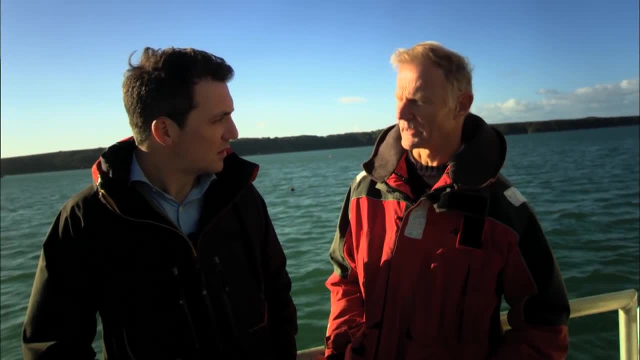 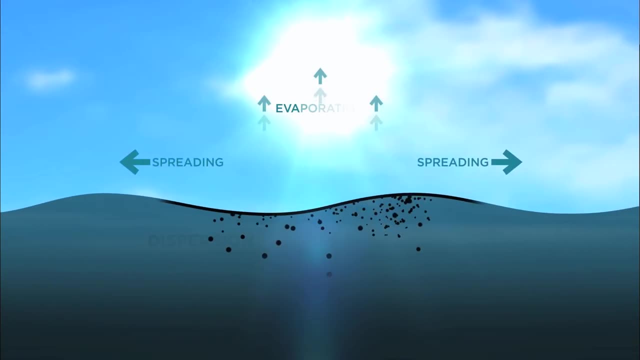 in our response. it will eventually get degraded by these microorganisms. We've seen that from the moment oil hits the water, it is influenced by processes. Some of them take effect immediately. others, like biodegradation, can take months or years. 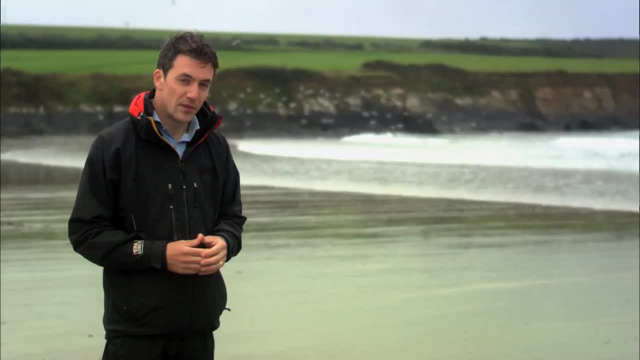 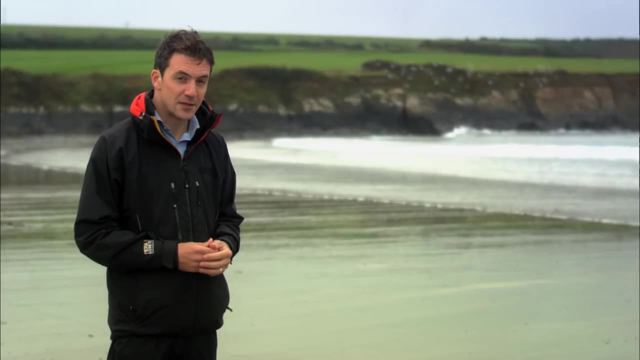 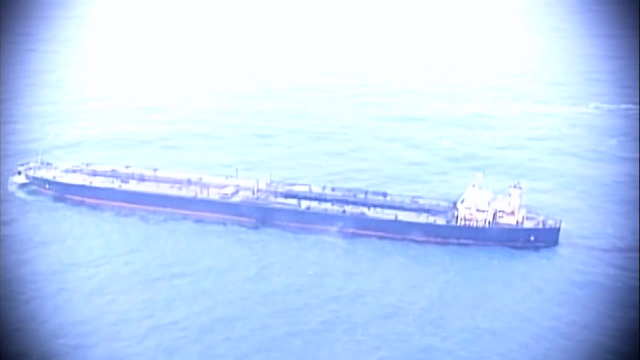 Understanding these processes is crucial. There are so many factors to consider, and yet the need to deal with spills quickly and effectively is paramount. We can never know when an oil spill will strike, but if we understand how different oil behaves at sea, then we can at least be prepared. 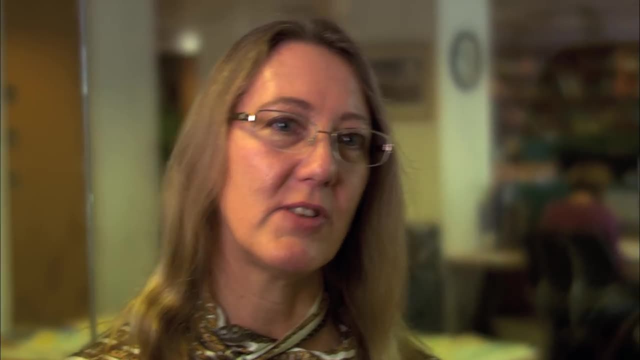 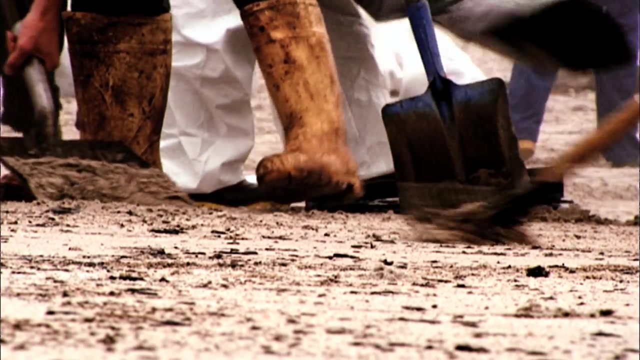 Planning is absolutely crucial. You can save precious moments right at the outset of a spill, when the damage is potentially the greatest. I think it's essential to know the oil that's been spilled, To know how it's going to behave. Forewarned is forearmed. 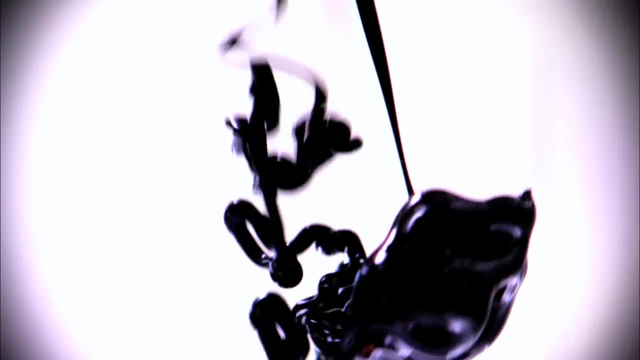 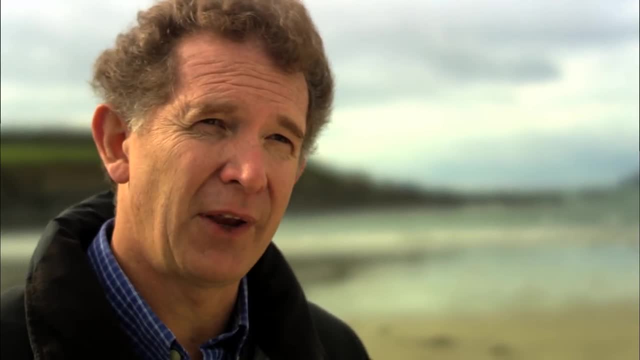 In military terms, it's know your enemy. Because different oils behave very differently in the environment, it's really important to know the advantages and the drawbacks from different techniques so you can tailor for that particular spill the right blend of techniques that will minimise the impact.